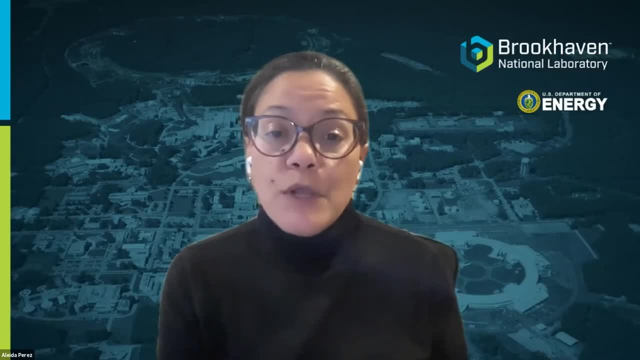 path that got them to where they are today. We hope that at the end of the 45 minutes, the information that you have heard will spark your interest in a STEM career and perhaps even consider being part of the Brookhaven Lab community. Good afternoon, I'm Aleida Perez. 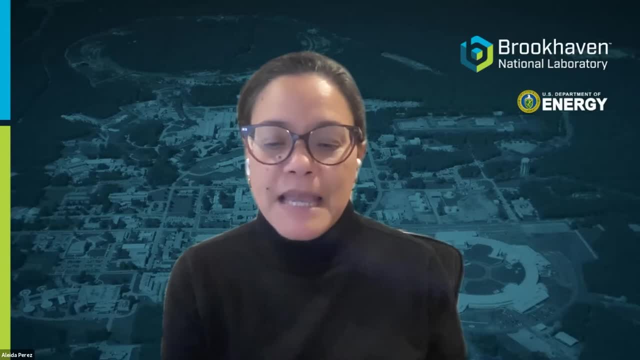 from the Office of Educational Programs here at Brookhaven Lab, and I'm joined by my colleague, Diana Murphy, who will manage the Q&A portion of today's discussion. Before we get started, I'd like to first introduce our panelists. I want to introduce our guest today. Just a few reminders. Please submit your questions. 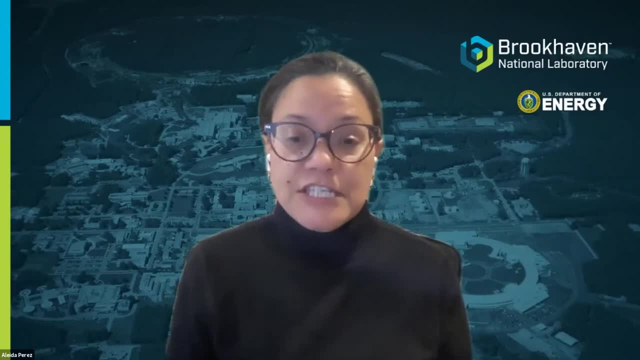 using the Q&A section chat. It's right at the lower side of your Zoom app. We will try to get as many questions as we can possibly can today And if you have any difficulties or issues with the video stream or audio, you can let IT know by making a comment. 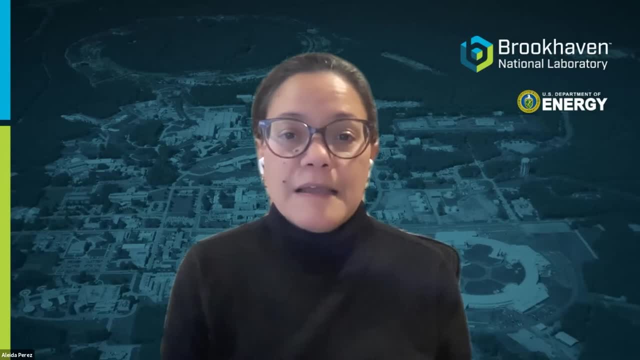 on the screen. If you have any questions, please let us know. And if you have any questions, please let us know. And if you have any questions, please let us know. And if you have any questions, just email us at email, a chat section. So today I am joined by Dr Oleg Major. 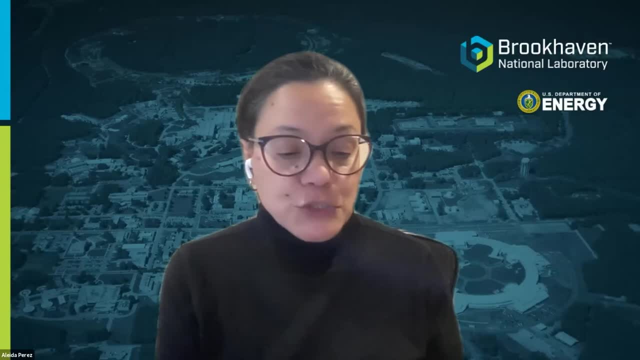 she said atmospheric scientists who recently joined Brookhaven definitional Brookhaven Lab environmental and climate science department and is the group leader for the aerosol related infrastructure group. Today, Olga will share her work on how a lot of aerosols impact climate systems. 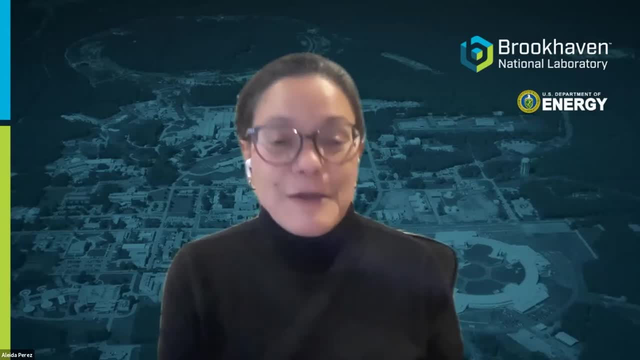 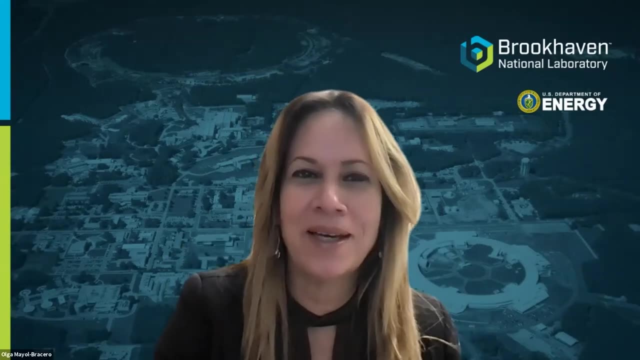 And also tell us about her career at Brookhaven Lab. Thank you, Diana. path Olga, bienvenido, Welcome. How are you? Thank you, Aleida. Good afternoon everybody. I am doing very good. I'm happy to be here. so thank you for the invitation. Awesome, I know. 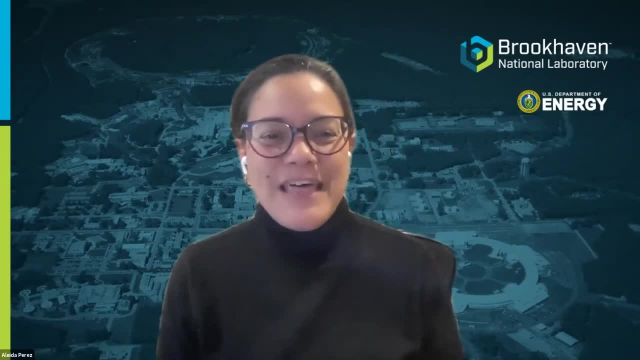 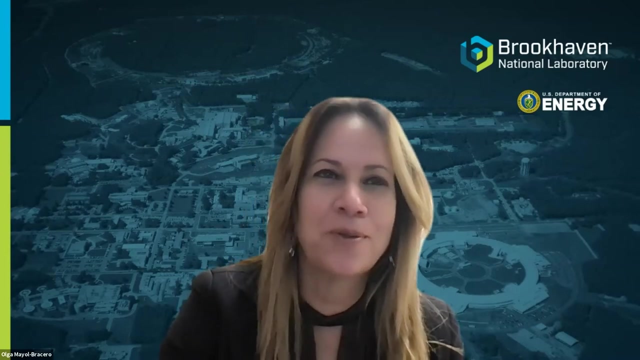 you joined BNL very recently and I know that we will talk a little bit about your career path, but where were you before you came to BNL? Yeah, so I joined the lab in August this year and I come from Puerto Rico, where I used to work as a full professor at the University of 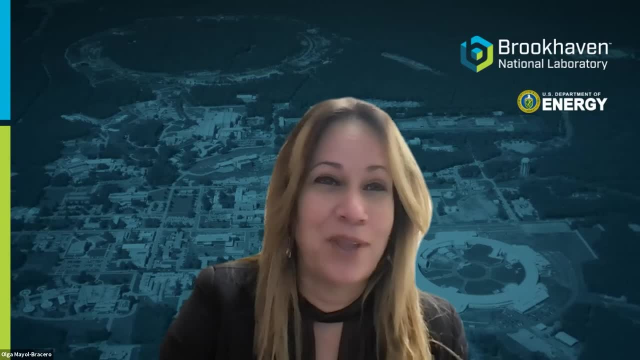 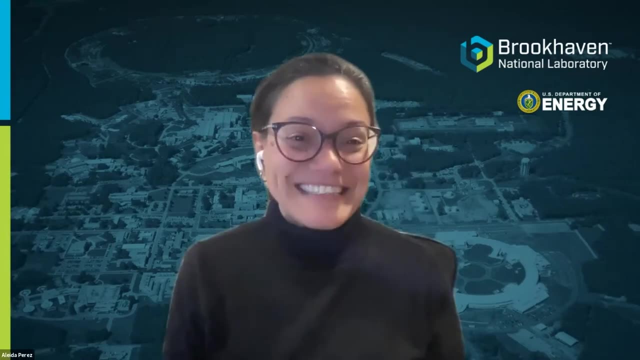 Puerto Rico, so I'm happy to be here today to share with you- you know, some of the work that we've been doing over the past years. Awesome, It's a very big but good change. It's a pleasure to have you here. It's a pleasure to have you at BNL, okay. So one of the things that when you and 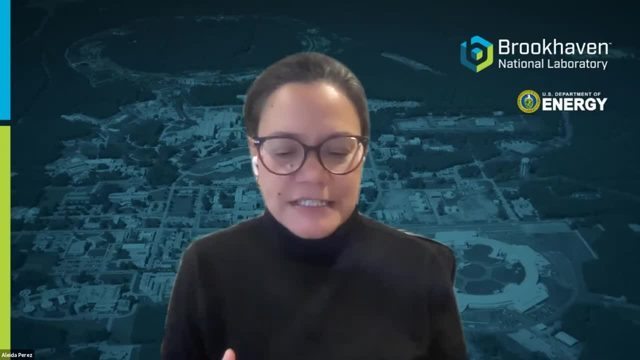 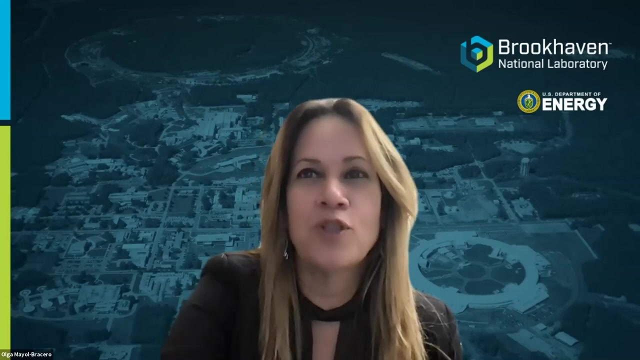 other atmospheric scientists and for our students and audience that we have today here. what is an atmospheric scientist? What is it that you are and you do Sure So? an atmospheric scientist is a person who studies the physics and chemistry of the atmosphere. So specifically, 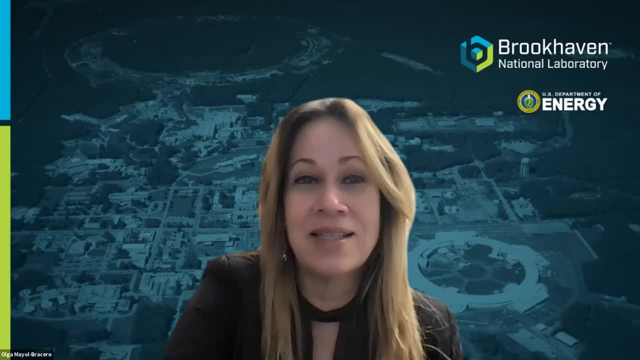 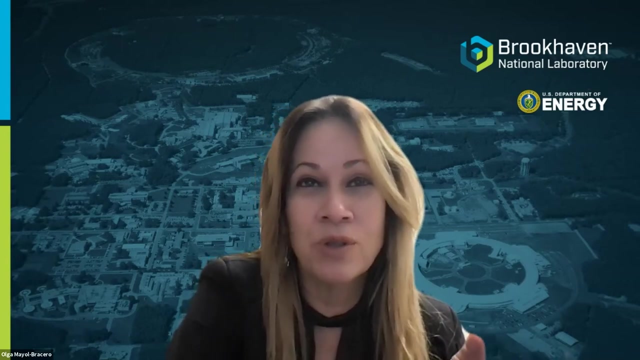 we study, for example, clouds, gases, aerosols, which are airborne particles, and we'll be talking a little bit more about those, And atmospheric scientists work in topics such as atmospheric composition, air pollution, weather prediction, climate change, climate. 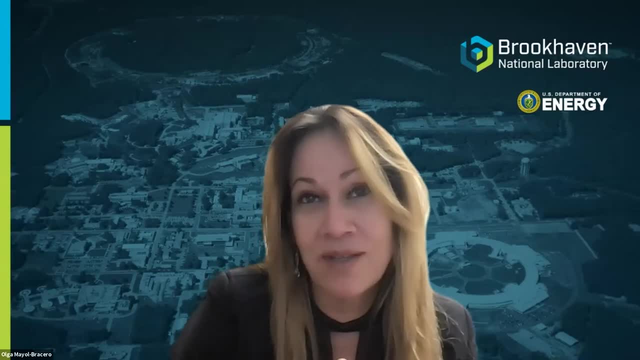 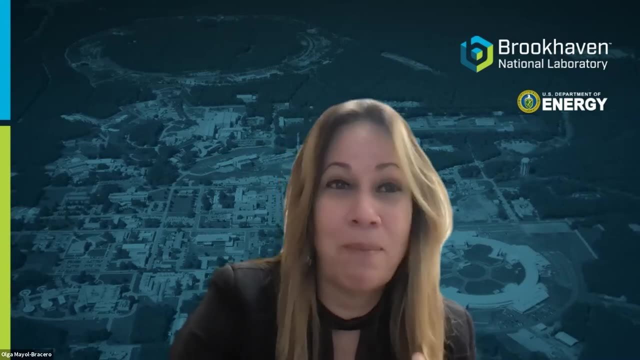 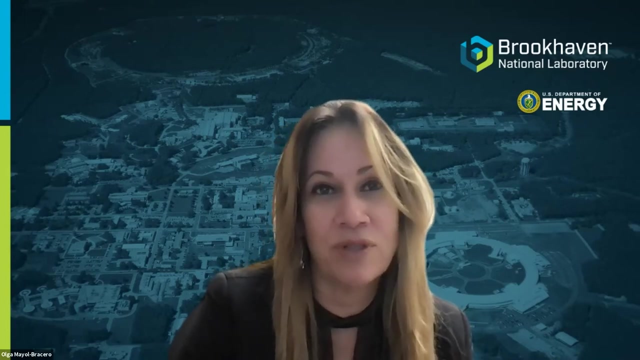 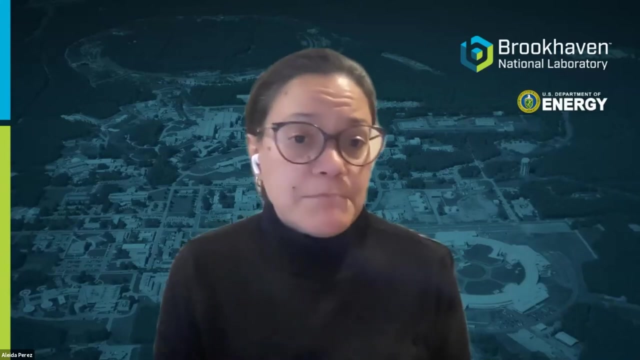 trends. My formation is in chemistry, so my PhD was in chemistry and during my postdoc I worked with atmospheric gas. so I've been applying my knowledge in chemistry in the study of atmospheric sciences. So I'm focusing on aerosols and on clouds. Yeah, So how those, for example, the particles that we 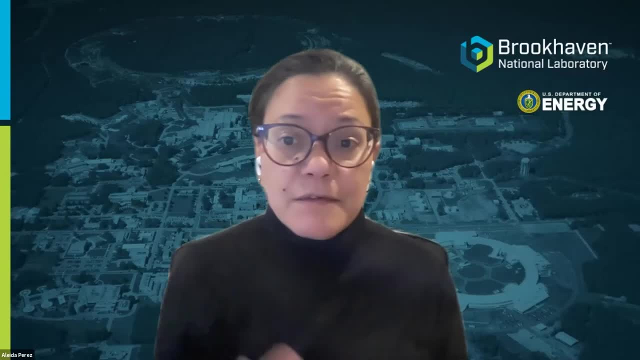 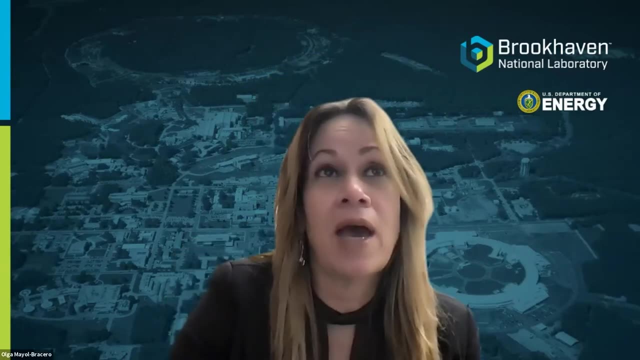 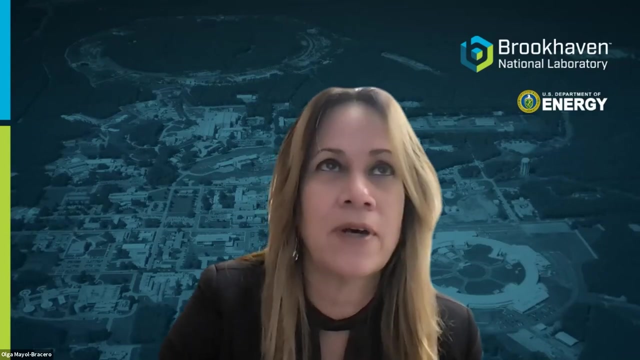 emit, the chemistry of those have an effect in the way you know. clouds just an example. Yeah, no, I could share my screen now and I could show people you know, if they don't know what aerosols are you know. let me see if I can do that quickly here. 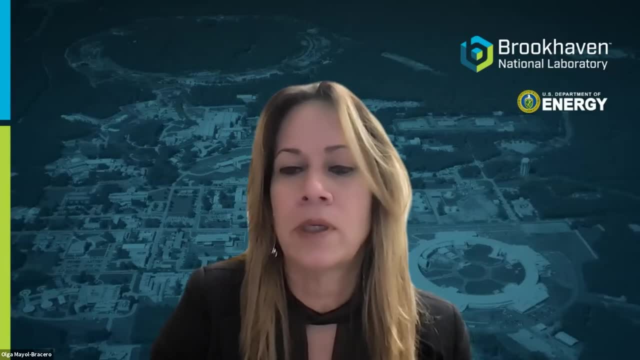 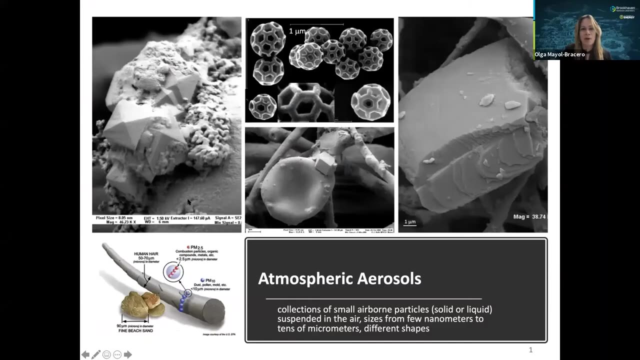 So when we talk about atmospheric aerosols, we are talking about these very small particles, that they can be in the form of solid or liquid, you know, and they are suspended in the air. And when we talk about those that are in the atmosphere, they are in the air, but you can have 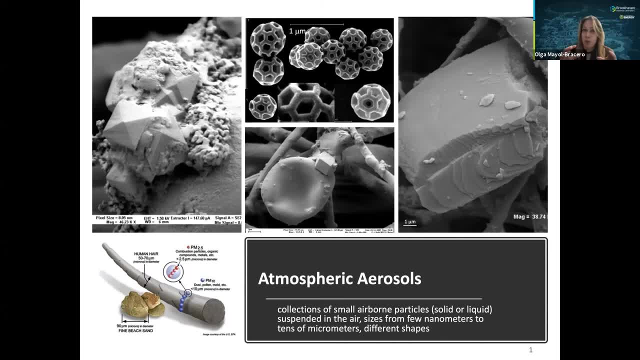 you know aerosols in a can, you know in different places, you know. but when we talk about atmospheric aerosols they are solid or liquid suspended in the air and you can see that the sizes they vary. you know you can have very small particles from like few nanometers to 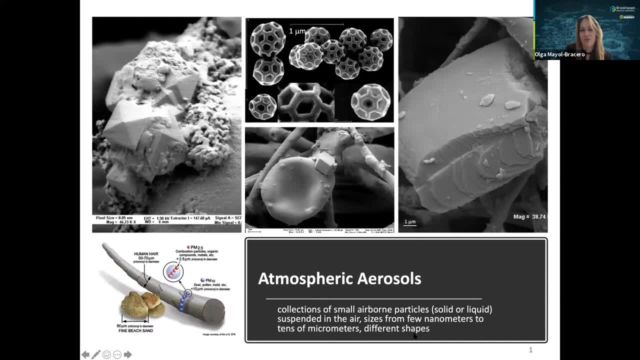 really large particles, that they can be in the tenths of micrometers, And those that you see here are images that we took using a microscope of high resolution, And you can see that they have different shapes. you know different sources And when you compare them, 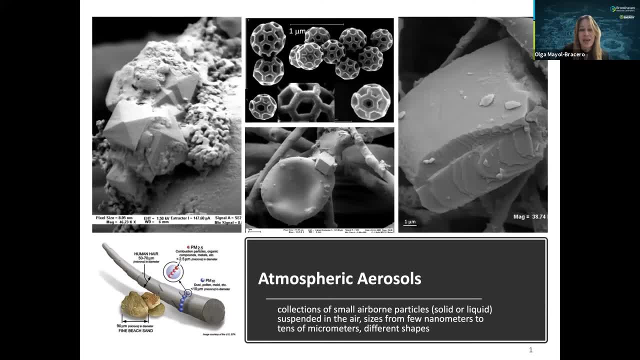 like what we're doing here with a hair, you know, a human hair. you can see, for example, here beach sand, you know, and here very, very small particles like those that are very dangerous for, you know, public health, you know, and they are really really small when you compare them with a. 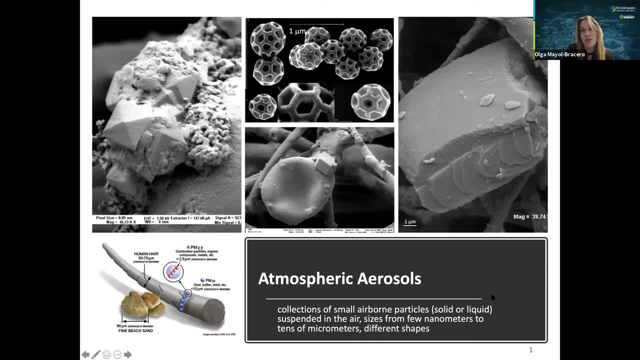 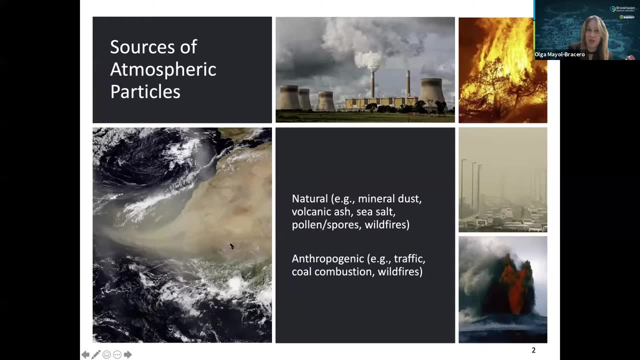 human hair. So, and those particles you know like people sometimes ask so, where do they come from? Do they come from the cans you know from, from aerosol sprays? Well, when we talk about atmospheric aerosols, they come from different sources and some of those sources can be natural, like 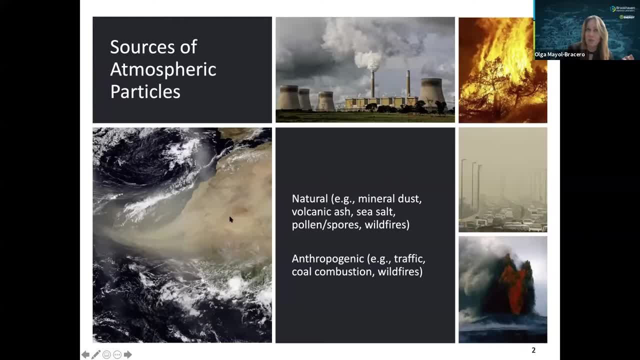 like from the desert in the Sahara, for example, in Africa, or or from volcanoes, eruptions, you know, like here, but they can also actually be anthropogenic, like from traffic, from cold combustion, from wildfires, you know So. so yeah, they have different sources as well. 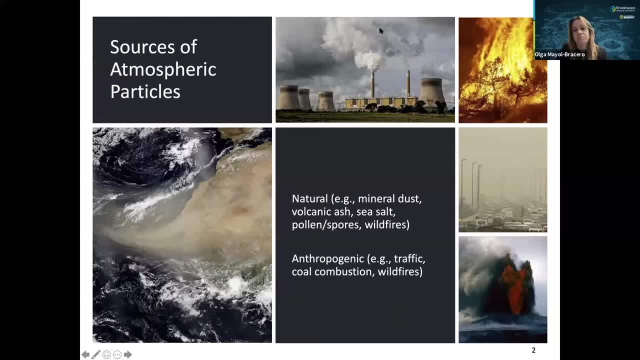 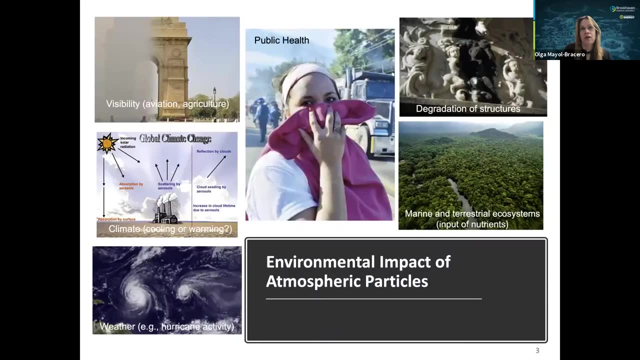 So they have different, different shapes and different sources of them. So, knowing that they are different sources of these atmospheric particles, what is the impact of those atmospheric particles on the environment? you know health, weather, climate, you know, Yeah, so I can, I can use these to explain a little bit about that. you know Part particles when. 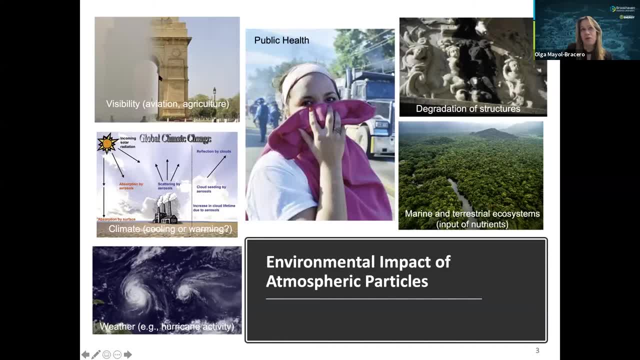 when they are in the atmosphere they can affect visibility. you can see here there is a indian gate in delhi and you can say: you, they, they over. you know close together these two images, you know these two photos, on a day with a lot of pollution and actually this was just after the lockdowns of 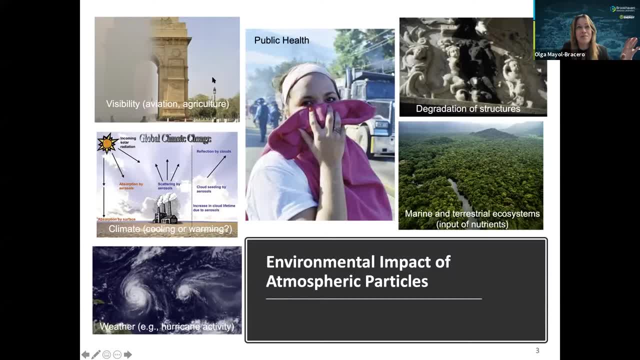 covid19. you know, at the beginning of the covid pandemic and you can see the difference. you know how can they degrade the visibility. and this degradation, invisibility, can affect aviation, agriculture, you know, can have different impacts. of course it's gonna affect public health, you know so. 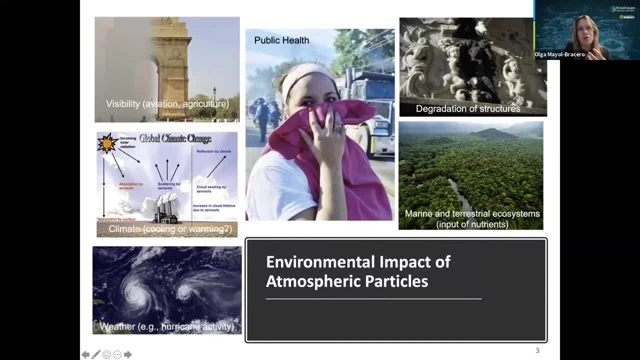 because of those very small particles, we can. we can actually breathe them and some of them can come inside. you know our respiratory system. they can degrade structures. they can also have input of nutrients that can affect marine and terrestrial ecosystem. they can have an impact on climate because they can. 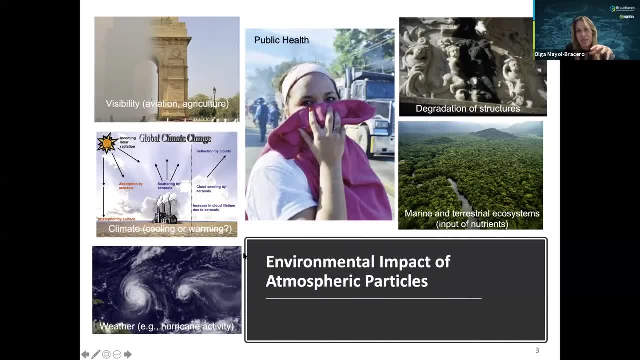 interact with the solar radiation as well as with the radiation that the thermal radiation infrared that the air is emitting back to space. they can affect that energy balance, you know, and that can produce cooling or warming of the atmosphere. and they can also affect weather, for example affecting the formation of clouds or affecting 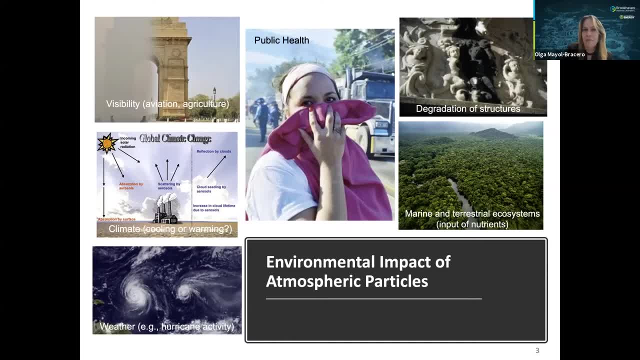 UV rays, etc. after 10 noon: slowly: Stupid, Birkinisa's, pastezuoc万子, CorBYN, раск, Brown, Rain, hurricane activity. so they have impacts and our group over the last years, while i was working in puerto rico, we focus on on these three areas: climate, weather and also air quality, which has 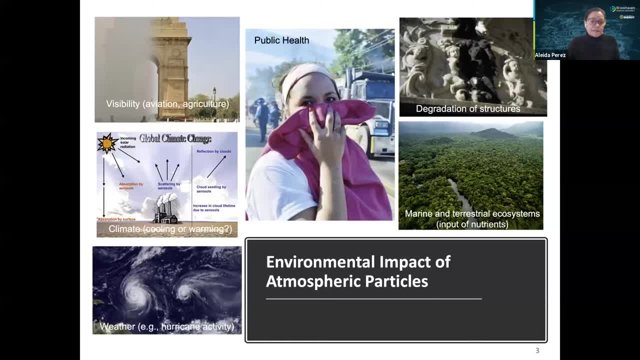 to do with public health and visibility? yeah, because you know the health quality, the air quality, in terms of the health right we hear about asthma and other respiratory illnesses that tend to be associated with the increase of this particles right, this increased atmospheric particles in certain regions and more you know affected. some groups are more affected than others. 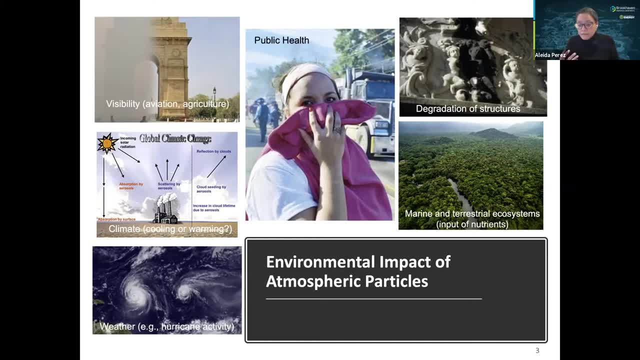 and usually, you know, nations that are, uh, that are not as as wealthy, tend to take the brunt of that, of that, of that as well. i remember when i was growing, puerto rico, the sahara- uh dust, you know, and every june you will see that coming uh on the island. 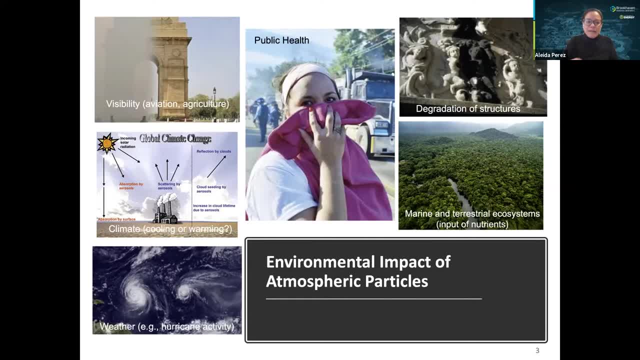 um, so i i know that you know you talk about the environmental impact and and and the health impact of this atmospheric aerosols has on on on the planet earth and also humans, you know. so what aspects of that you just sort of: why should we care? why people should spend, you know, pay attention. 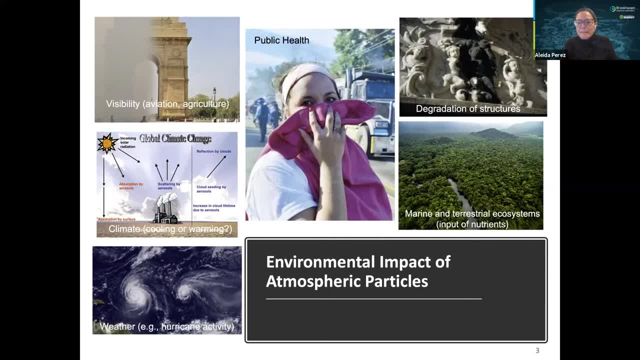 to, to to this science. well, precisely because of that, you know the, the impacts that, um, in the case of the science that that we were doing in puerto rico and also we are doing right now here, uh, the, these particles, they, they can have an impact in the on the environment, and we should. 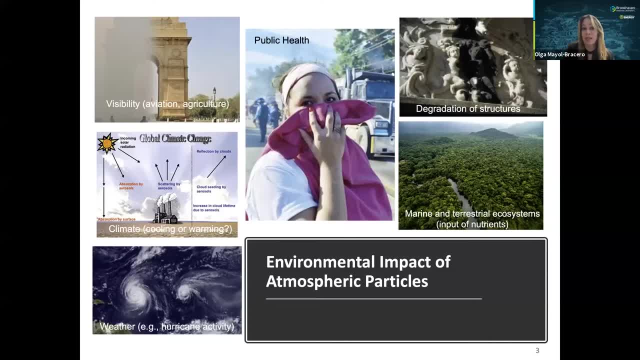 care about our environment that can produce not only damage to ourselves, but also to nature, to animals, to structures, you know, and to things that affect us, such as climate and weather, for example. so we really need to to to care about this and and uh- yeah, you will see what we've been doing- uh, over the years, uh, 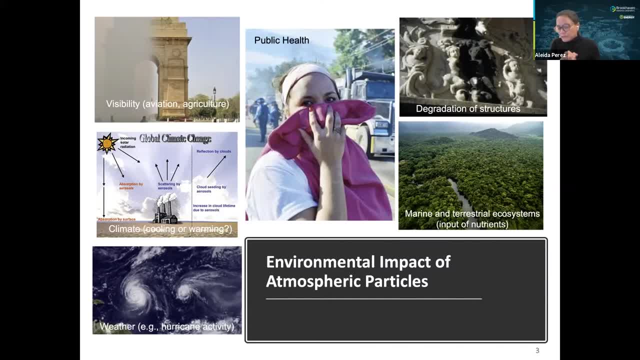 so now that you mentioned that, you know that in puerto rico, and that's where you were before you joined us here, bnl, um, you were you as i was reading and we were talking. you were the director of atmospheric chemistry and aerosol lab. so can you tell us a little bit about the mission of the? 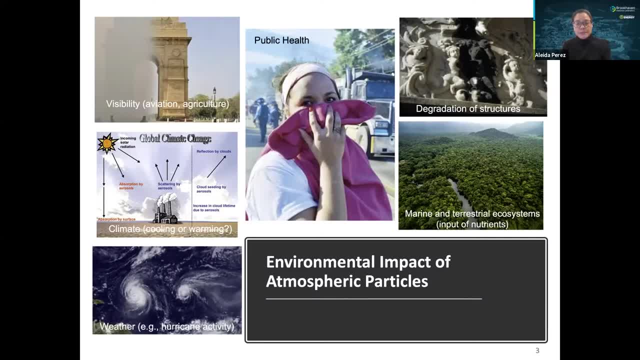 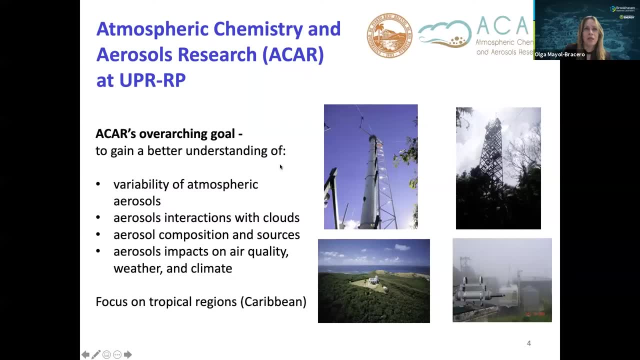 research mission of your, of your, of your lab back in puerto rico. yes, so let me show you here, uh, the, the group that i had at the university of puerto rico, who i was leading. i was working in the department of environmental science and, uh, we were lead. i 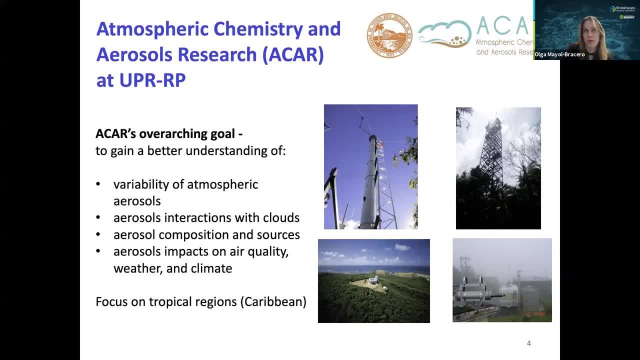 was leading the atmospheric chemistry and aerosol research group and uh. the main purpose of this group was to gain a better understanding of the variability of atmospheric aerosol, so temporal, and variability also of aerosol and cloud interactions. how can aerosols impact cloud formation, for example? also the composition of these aerosols and the sources. where were they coming from? 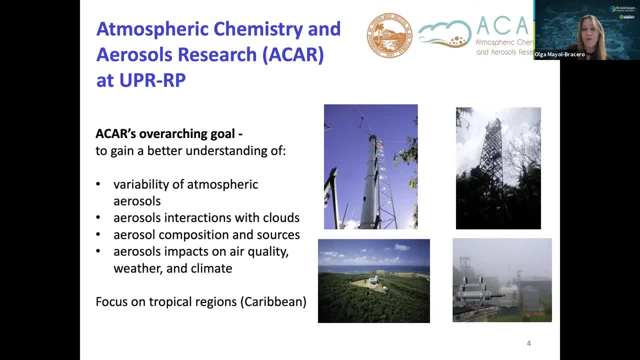 we, for example, we studied a lot- we were talking about african those and mineral does. we studied, put a lot of effort and a lot of time, you know, on trying to understand better the impact of those in the caribbean region. and also we studied biomarkers, burning aerosols, sea salt aerosols, anthropogenic aerosols and the impact of those on air quality. 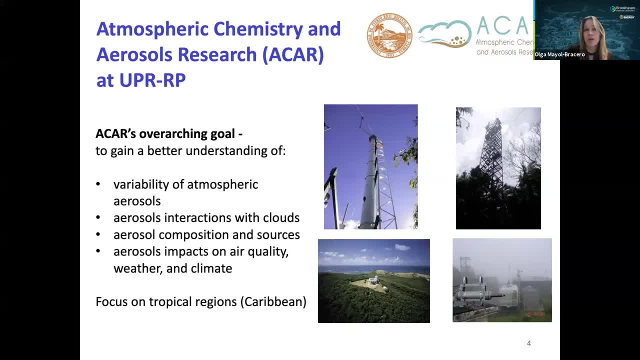 weather and climate, And most of the work that we've been doing was in tropical regions and in the last years we were focusing in the Caribbean. Yeah, that's very, very and I think we will talk a little bit later about the impact of that. but so you focus, you. it was not just 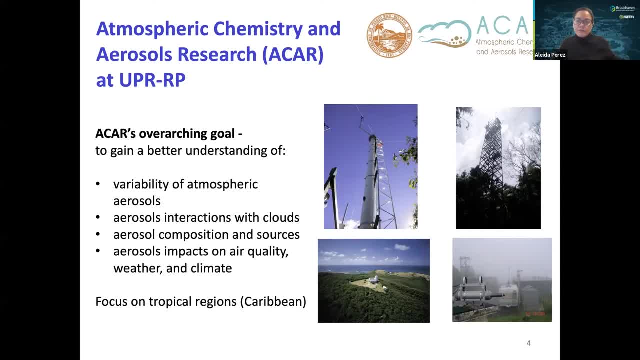 in Puerto Rico. right, it has a broader impact to the Caribbean region as well, and so so it had that had that level of impact as well. When you- you and I were talking about you also mentioned that you were the director. you were the director of two atmospheric observatories. 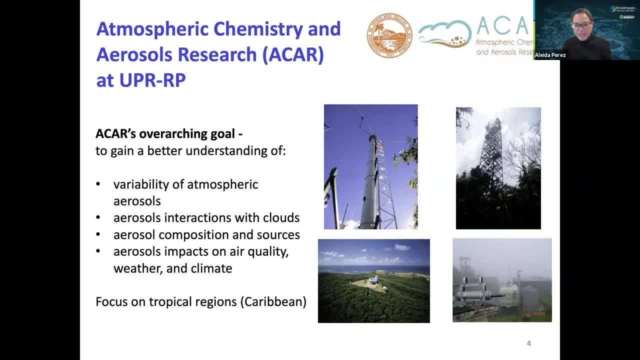 Can you tell a little bit about the, about you know about that work and the and the findings that you've been working on? Yeah, I mean, I think you know, I think you know, I think you. 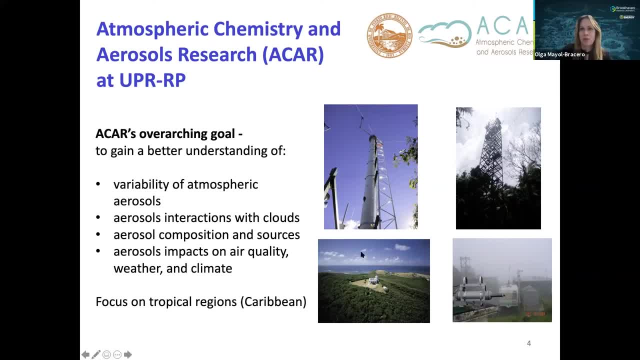 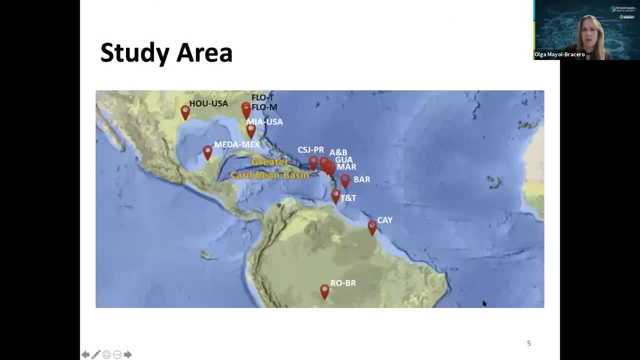 you, you had, Sure sure, actually, those images that you see here. they are from some of the observatories. but before I get to the observatories, let me let me tell you something else as part of of, because this is going to lead us to why we had those observatories. 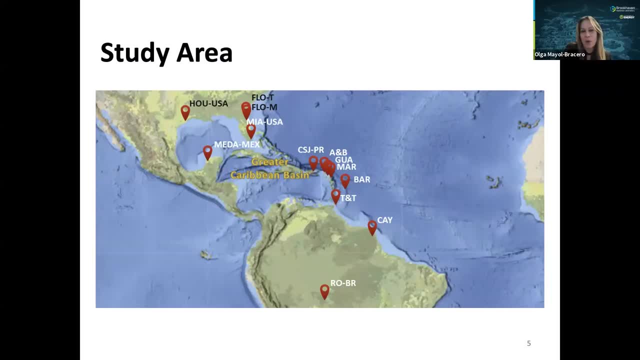 where we had them, you know. So, so, as part of my work in Puerto Rico we were, we had several projects in the tropics and this map here shows you the locations of those projects and they, you know, we had the, The landed object, and we had the water. 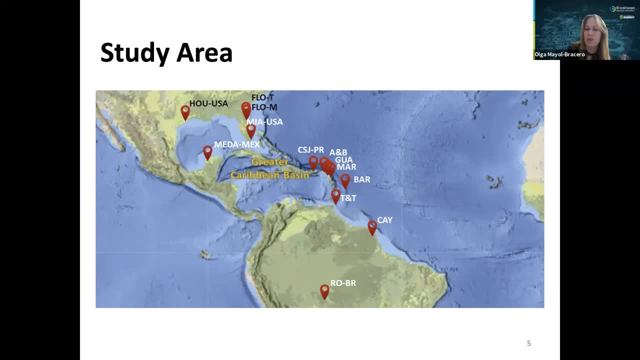 So in the last year we focused more on the greater Caribbean region And and it was not only because this is where I was living, but it was also because that region actually it's. when we talk about, about the Caribbean, We're not talking right now only about the Caribbean islands, but the 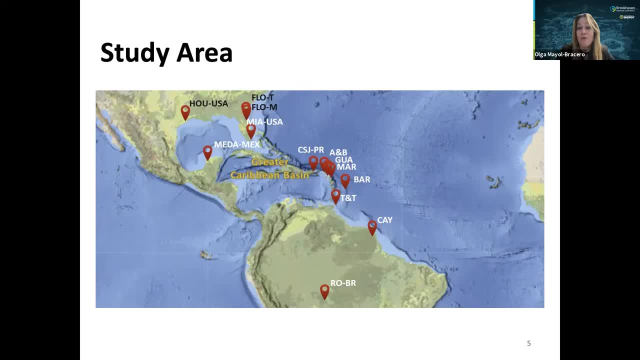 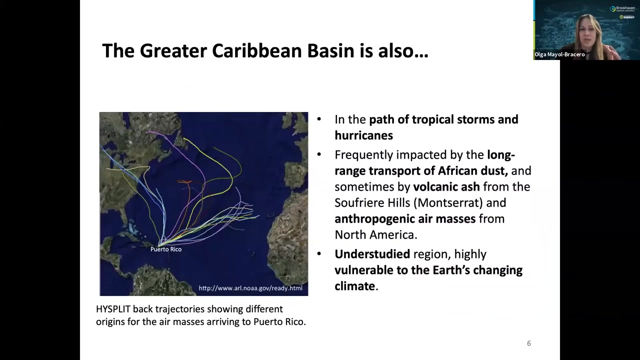 greater Caribbean basin And this is any country with coastline on the Caribbean basin. So we're and the processes that we study there. they can be applied to other regions in the world, but also also and that region that we have interest in. it's in the lie. it lies in the path of tropical storms. 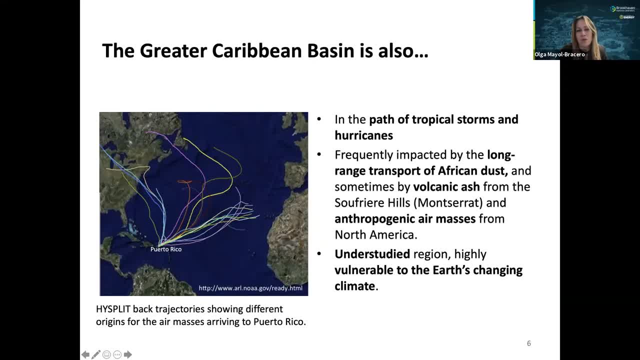 and hurricanes, because you know that a tropical storms and hurricanes they form in in this area, here in this region as well, is impacted by african dust, as we mentioned before, but also we have here the sufrier hills, a volcano in the island of montserrat, and also we get sometimes the impact. 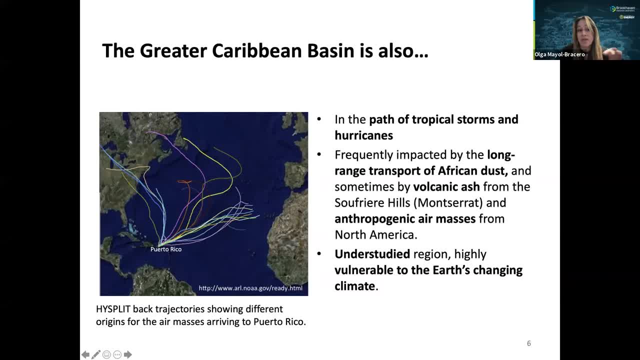 of that and sometimes, as you can see, by these trajectories of air, air mass trajectories, that is, these lines that you see here. sometimes even we get air masses from north america and those also bring some pollution to the island. in addition to that, this is an area that is understudied. 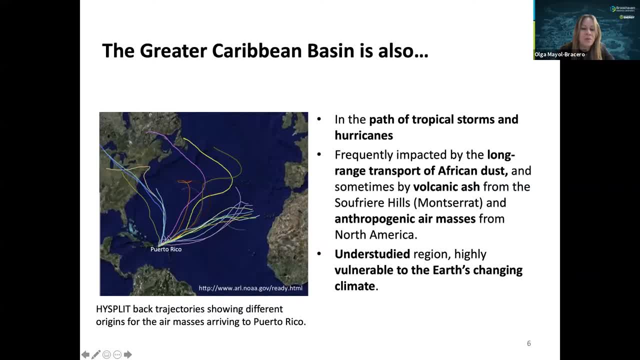 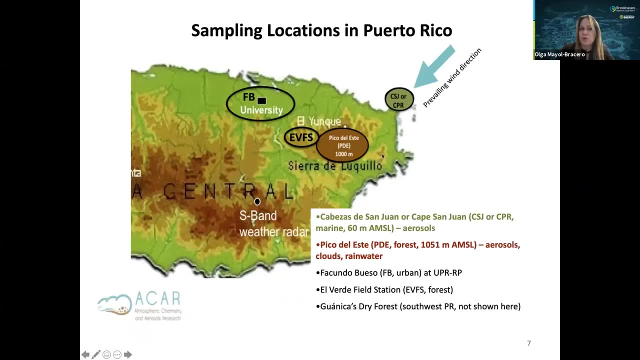 and is highly vulnerable to the earth's changing climate. so those are some of the reasons why we decided that an aerosol monitoring program was going to be important in the region, and that's why we decided to have some stations in in puerto rico and we we put one of them here in the northeastern tip of the island and the 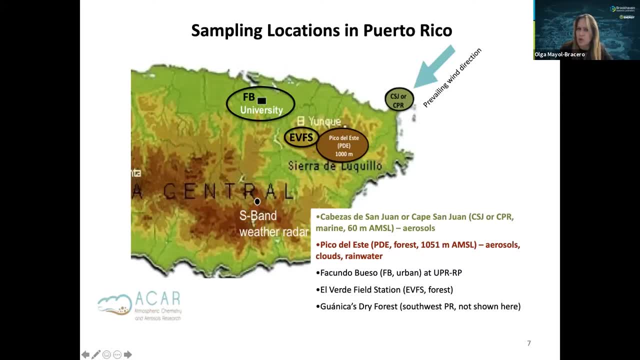 other one. the other main station was here. we we also had other places where we we've been doing measurements, but these two are very important because they are not located on the same area. so we have to recognize that the location was strategically chosen because the prevailing wind direction that we have is northeast, you know. 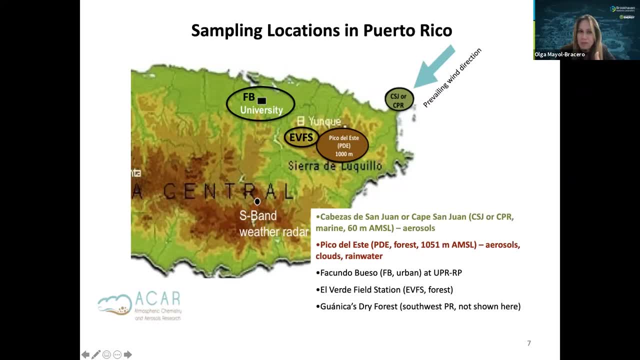 so here we were getting a. this station is called cape san juan. we're getting very clean air masses that only has the influence of the ocean, or sometimes even sahara and those. and then this station is in a cloud forest, so it's high and there are clouds all the time, but then we can see. 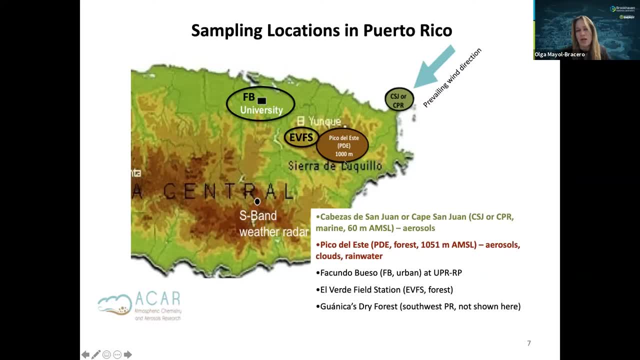 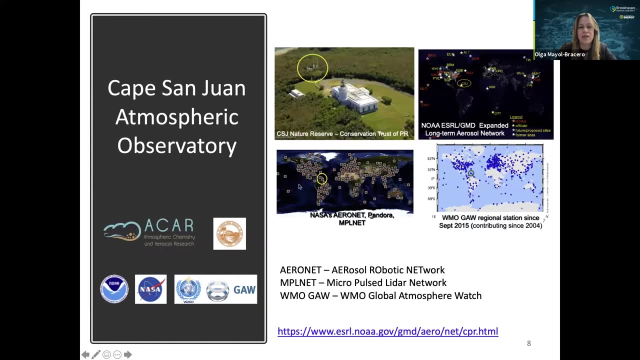 so that they have passed this station with the clouds that we have here. so the two stations are, you know, in an excellent location for aerosol and cloud studies and these are the stations. you know. this is the one in the coastal side and we're part of, uh, we're in a nature reserve, it's a. 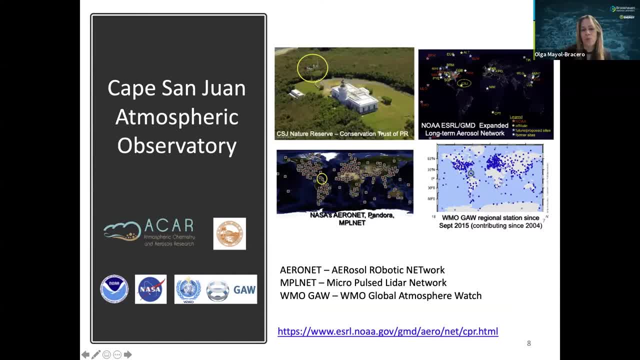 beautiful place where there is a lighthouse, and we are part of the NOAA aerosol network and also part of nasa- nasa's ironate and nasa's pandora and nasa's mplnet. so these are all networks that nasa has to study aerosols and also we are part of the world meteorological. 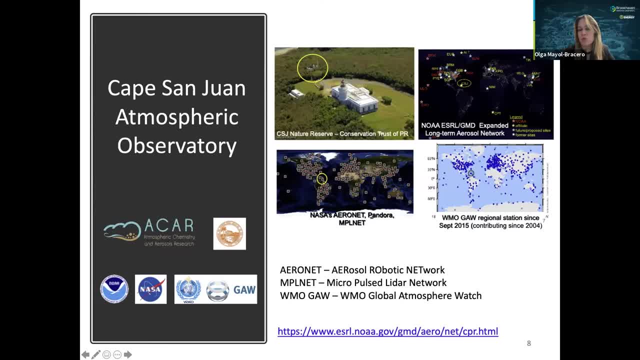 organization. they have a program that is called global atmosphere watch and our station is also part of of these and we've been running 24: 7 since 2004. except for the impact of maria, that will do. and this is the other station. it is also a beautiful place. it's located in a national forest. 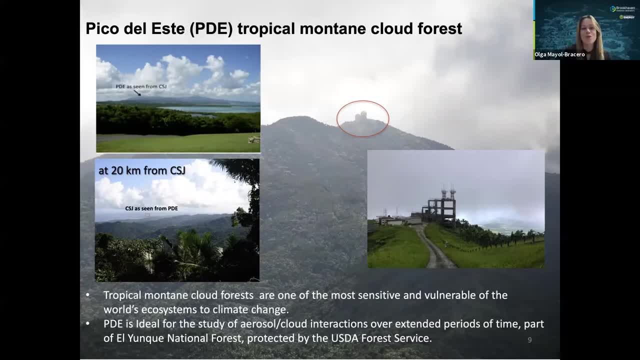 you know that place, is it? i know that place is called the name of this rainforest and it's a cloud forest, as i said before, and it's an ideal place to, to, to study, you know aerosol and cloud interactions, and it's a mountain, it's a tropical mountain cloud forest, so it's one of the most sensitive and 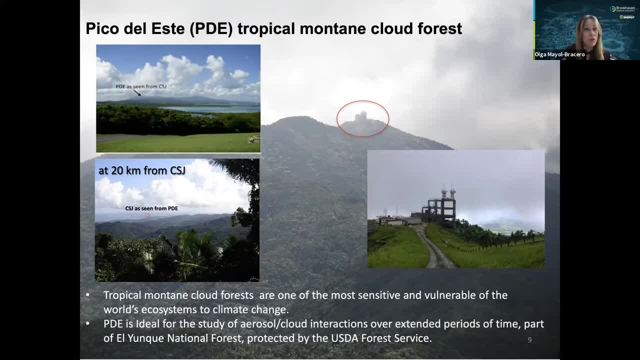 of the world's ecosystem to climate change, so it's also very important to understand what's happening in this, in these places in particular with, for example, a what has to do with cloud and the impact of aerosols on cloud, because that could impact the hydrological cycle. 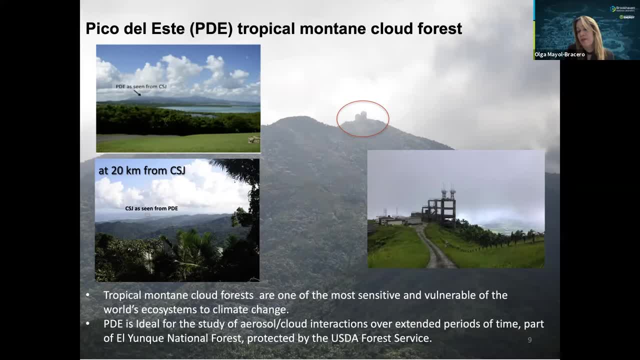 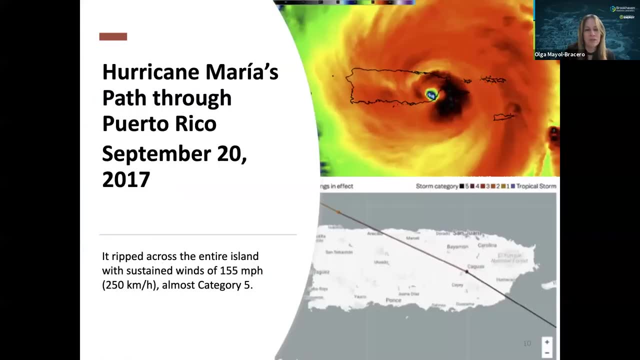 so, but i don't know. i think that maybe maybe some of you know that that we were in 2017. uh, we had the impact of hurricane maria in puerto rico and, uh, it was a very strong hurricane and was almost category five when it hit puerto rico and it ripped across the entire island. 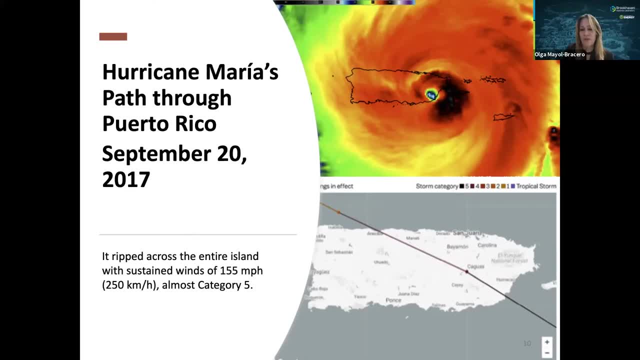 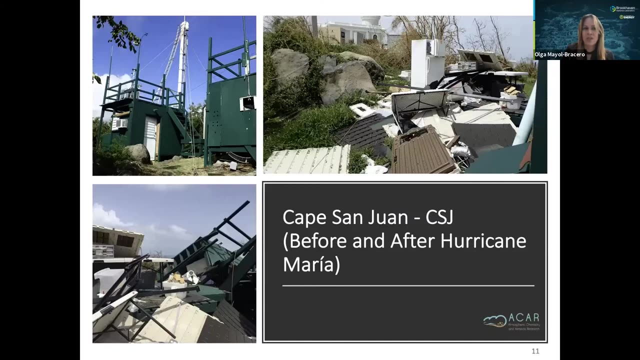 the winds, as you see there, they were over 150 miles per hour and it has been the most powerful hurricane to hit the island in almost 90 years and it devastated the island, but also it devastated the ocean, or thełuIt is one of the reasons, uh, uh, hey, often people think about like it was um. 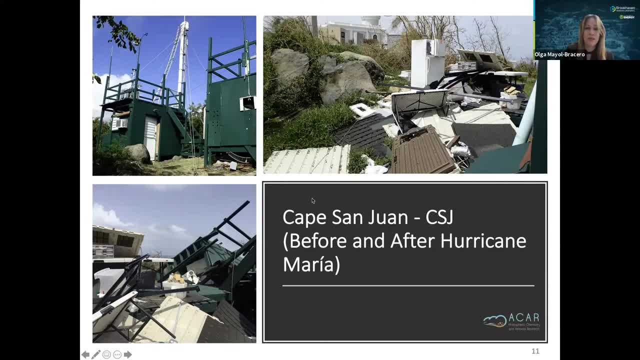 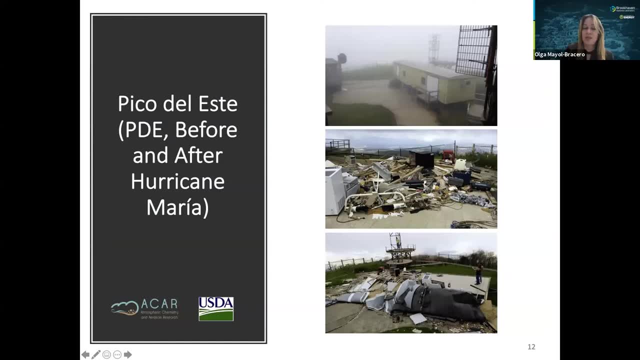 uh, it, let's say, one ocean and it wasbad, was really bad�, believe, but it was. it hit like a million people, you know, and it was like a great deal that really a lot of people had. however, the tides were low. Central Ocean was very high, right, like it was, uh, uh, very, very high. so 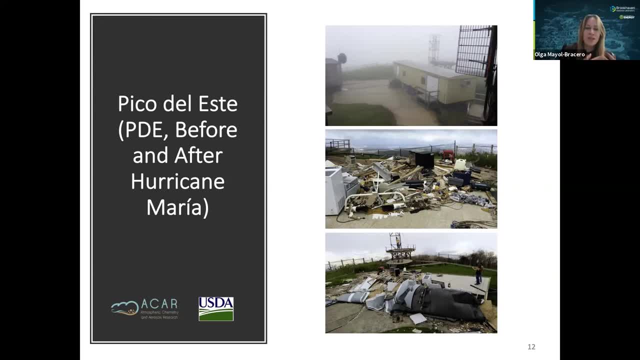 that's why they did world class American water studies earlier when they started to go to uh. for things like this happen in life. you, you, they strike you. you know, you, you have to to think, you know. so now, like I was thinking, now what you know, I mean I've been raising this for 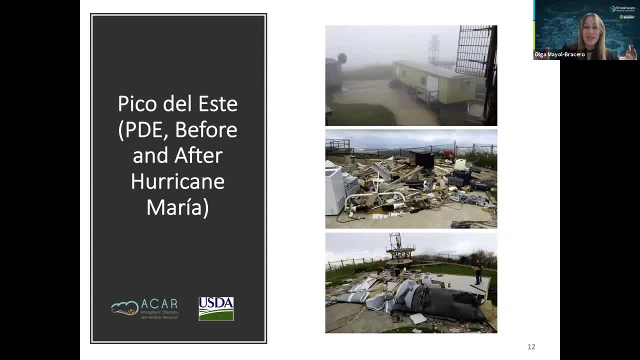 15 years and it's been destroyed in in, in seconds, you know, in minutes, in hours, you know. so what do I do now, you know? shall I change, you know, my job, or, or, or I start all over again, and you know what I decided. okay, let's do it. let's do it again, you know, let's start all over again, because with the 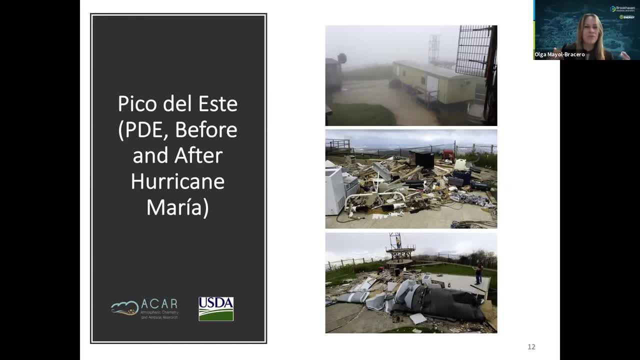 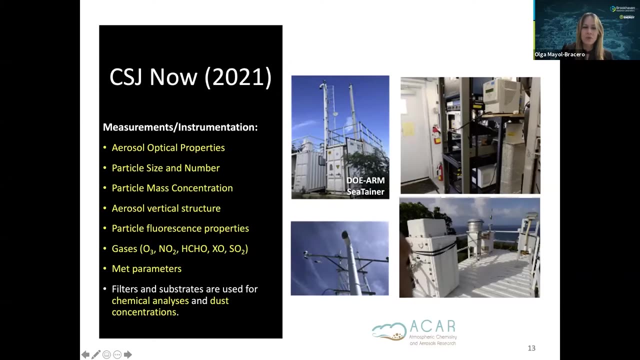 experience that I have and the help of the collaborators that I have, we should be able to be something better and stronger, and that's precisely what we did. you know, this is the way the stations are right now. we have two trailers there, and actually one of them was from a 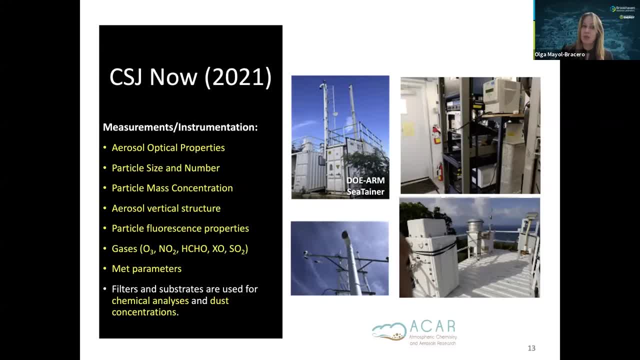 we arm. so the department of energy and the atmospheric radiation measurement program, we wrote, I wrote a couple of proposals to to get funding to to reconstruct and one of the proposals was this one and you can see that we are doing a lot of measurements there: the station. 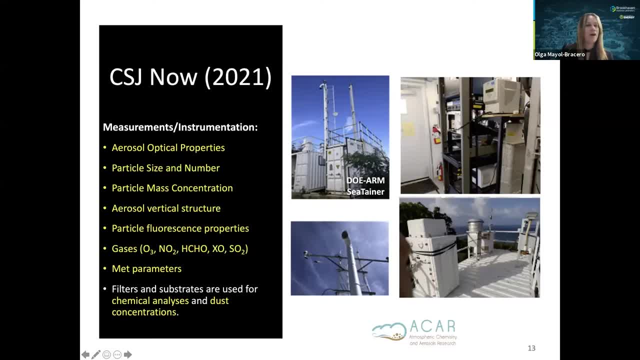 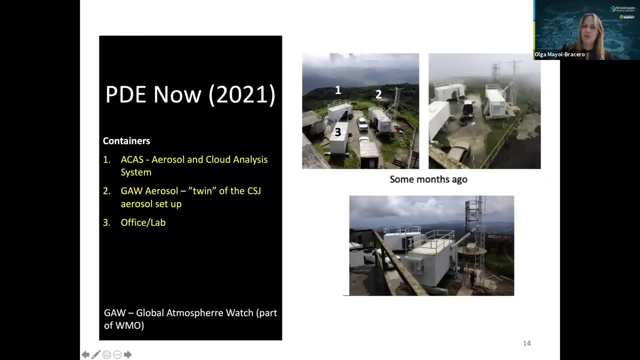 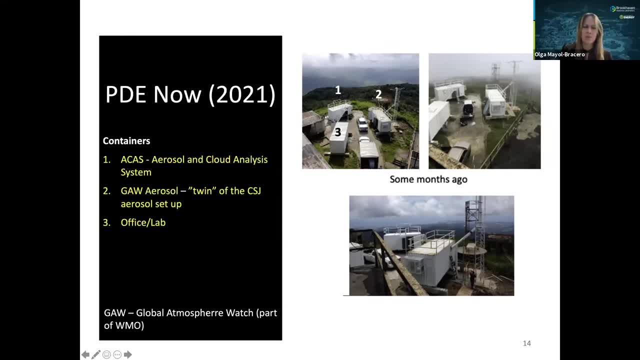 station still, but the station is a more robust and we much more capabilities that the ones that we used to have. so, like that saying, you know that we have heard so many times when they go and get tough, the tough get going. you know. so if we fall, we, we, we get to have to get back up. you know. 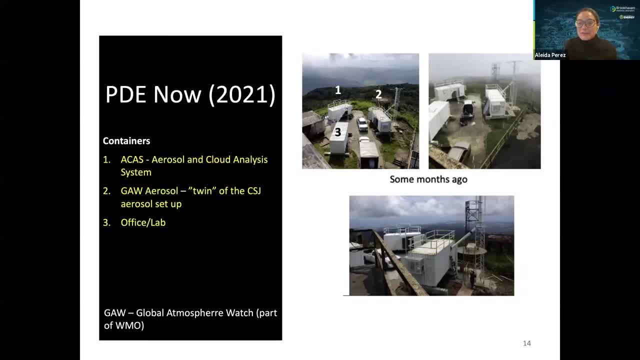 so I actually, like I I was going to ask about the, the. you know the rebuilding of the structures, because they, they look quite impressive and and and I just said, some looks uh, the, the equipment is better than it was before, right, so you are able to collect more precise and and and you know better. 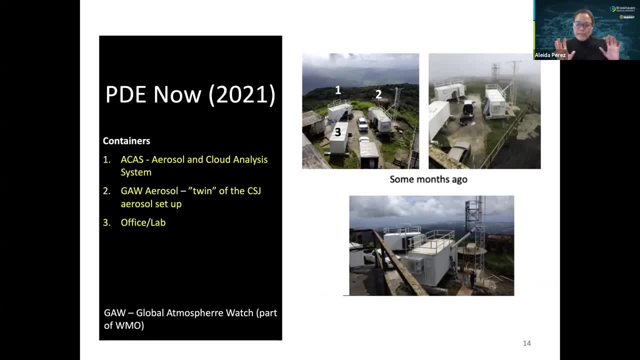 data, so do you- I? I do have students out that are state how that the data gets. you have people that goes to those stations to maintain them, or that's something that, uh, how often did that happen? yeah, yeah, you have to. you need to have someone going at least, at least every week. you know, once a week. 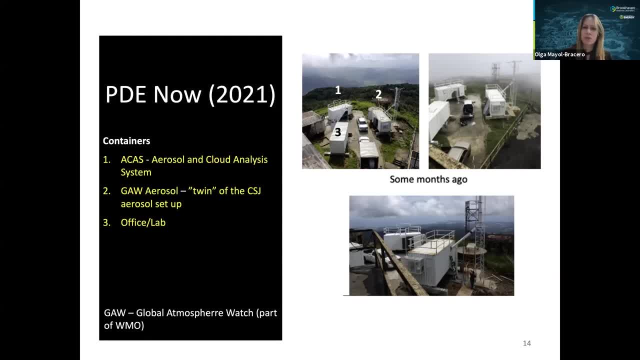 but the the good thing is that it's pretty close to to to the campus of the university is uh less than an hour drive. uh to to each station, you know. so if you going to see us to to the costar station or to the cloud forest station, to both of them it's, it's only, it's less than an hour drive, and uh. 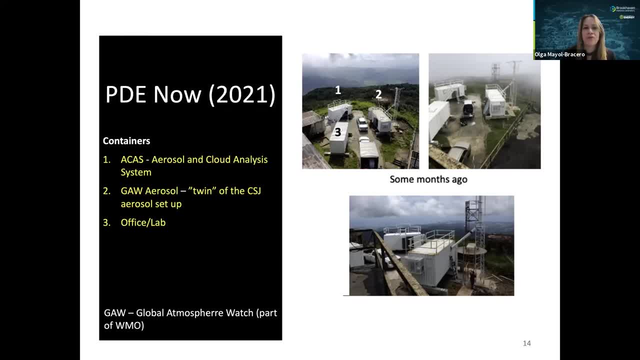 are, uh, but we still need, with the most students have, uh, you have to keep the instruments running. So, because we are doing research projects, but also we are providing data to other people, you know so, to other groups, you know, with the World Meteorological Organization, with. 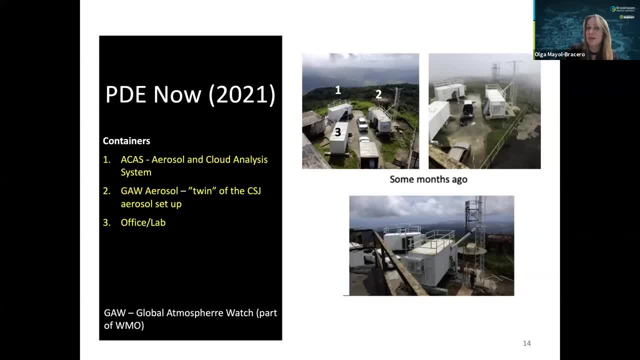 NOAA with NASA, So people are counting on those data. So it's important to keep the instruments running And when an instrument is down then you have to. if you went on Monday but the instrument went down on Tuesday, then you have to go back again, probably Wednesday, you know, to try to. 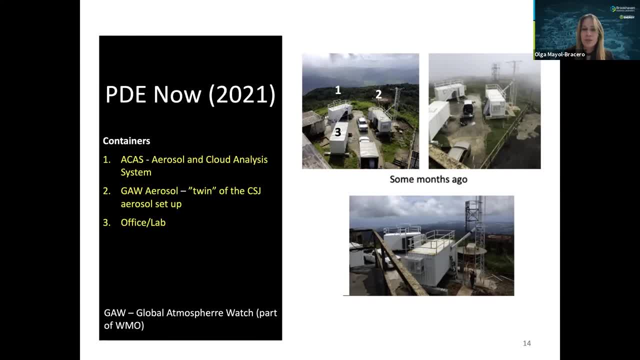 fix that instrument. So there are students, undergraduate students and graduate students, and there is also an instrument specialist in charge of this, you know, and the students get involved with the projects and with the instruments as well. Except, so say because you know, do you have the? there was a rebuilding of these stations. 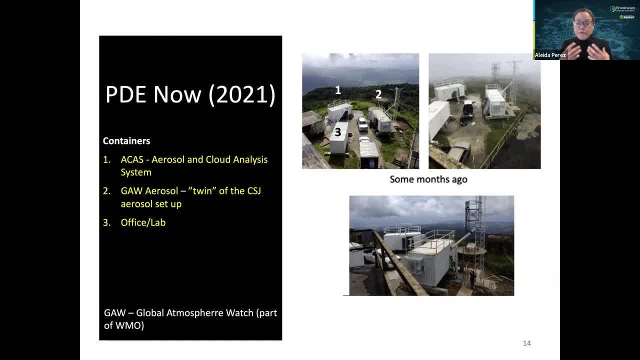 You are- I'm assuming you're still, you know, keeping the focus of collecting the information that we're, that you were collecting before, Maria, but any upgrades or any other type of information that these stations now are collecting, that is coming, you know, because of the upgrade. 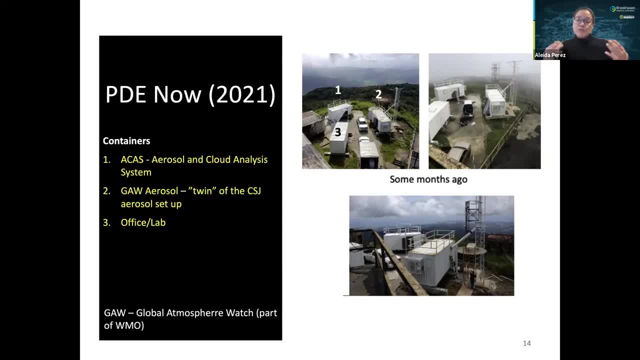 and the, you know the changes in climate and so forth. that allows you to collect a different set of information and to have you know and then gather information, gather a different perspective of the, of the, of the different areas. 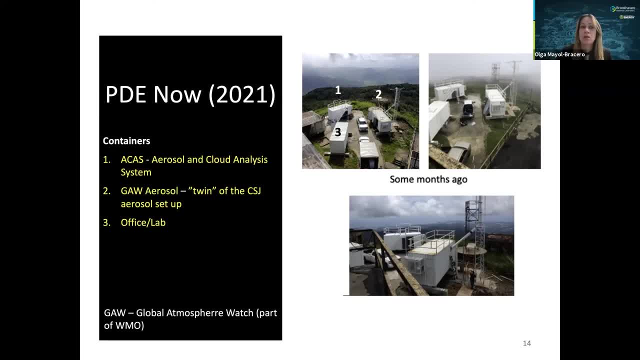 So you know there are, there are. I mean we, we managed, we have, and this is what you're seeing. here is a. it's a very good example. you know, one of the proposals that I wrote at that time was: 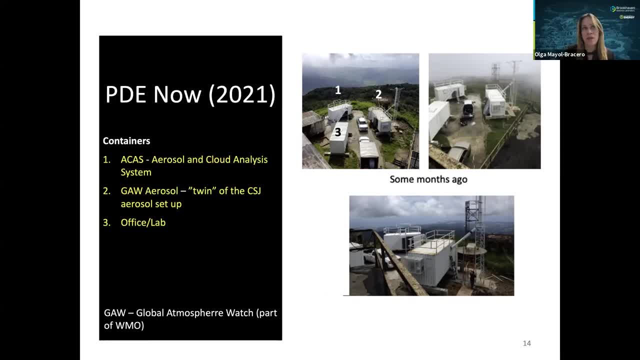 a proposal for NSF. They have a program that is called Major Research Instrumentation and this is a program that that fund ideas of, for example, development of of new instrumentation. So we propose to do the aerosol and cloud analysis system. 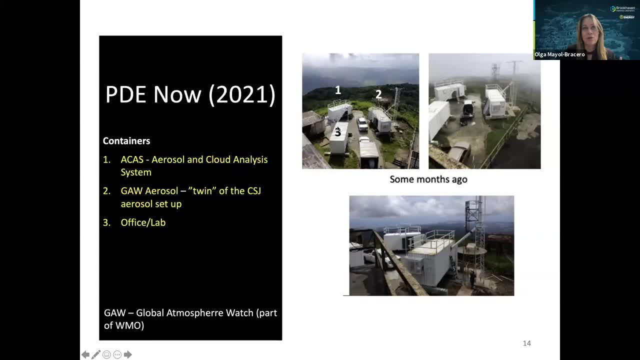 and this is this trailer that you see here. number one is precisely that. This is: it's a trailer that is going to be dedicated to the story, to the study of aerosol and cloud interaction, and it has seven different sensors that we did not have before. that they will all. 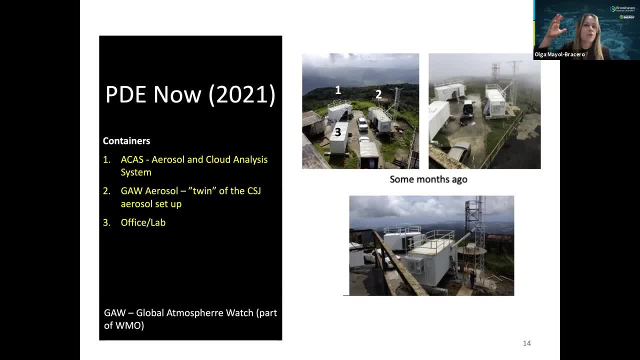 be connected to an instrument. So we have a very good template that will be able to sample cloud and aerosols and we will be able to get a better understanding of the composition and interactions of these cloud and aerosol particles, you know. So it's it's a good example of how, and that you know that proposal was. 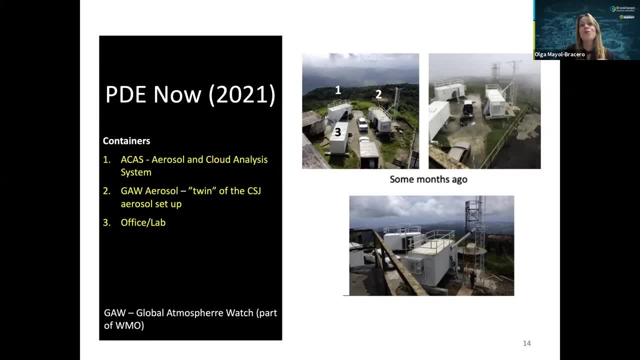 just 1.4 million dollars, you know, to be able to build this, you know. So we have a postdoc who is working on it, working actively in this project. very nice, very nice. just to the audience you're welcome to, uh. 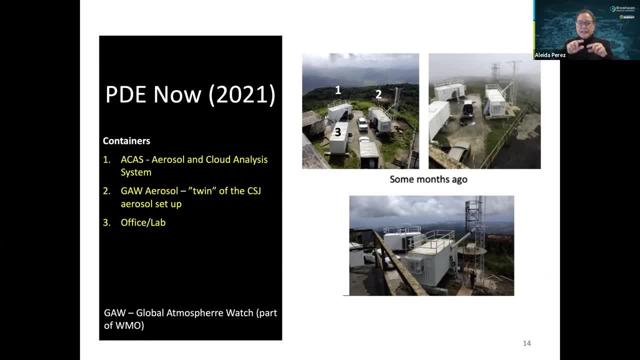 and put any questions on the q a uh chat. you know icon and uh, we will be glad to to, to, to answer them. um, so i i, one of the things that you know you, you mentioned as well, was that i know that were a professor at the university of puerto rico. uh, what kind of research is? um, what kind 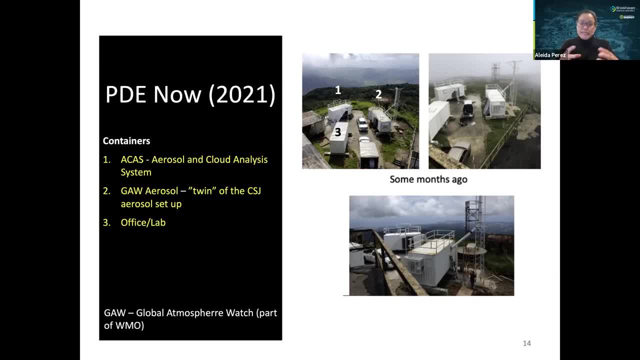 of research did you do? there is this, was this. you know, i know what's related to, to, to the acar project. in any other uh aspect of the research that you were doing that was very specific uh to the university of puerto rico and your research there. yeah, so one of the things that uh a very 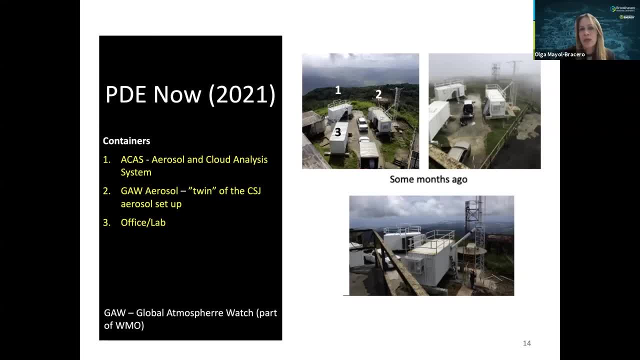 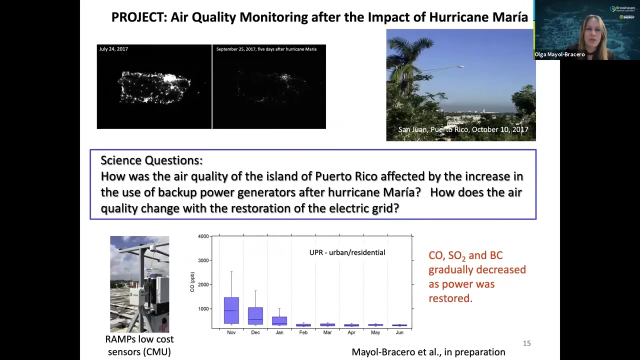 we had different projects and some of them were related to air quality. you them, we actually got the idea and wrote the proposal and got the funding for that and some of them were opportunities that they emerged. you know, life was what happened with hurricane maria. so i want to tell you a little bit about this project. uh, this is the project that, um, that was. 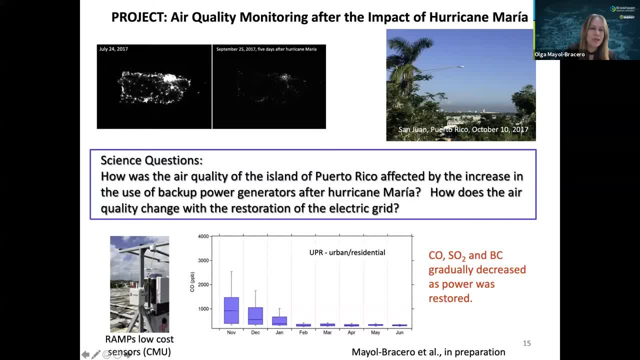 one of those you know. uh, this is the island before maria. this was july 2017. and this is the island before maria. this was july 2017. and this is the island before maria. this was july. This is an image of a satellite showing the island at nighttime. So you see the lights, you know, of the island. Now, of course, this is San Juan, where the capital is. So you see all these, you know, I mean, this is where the metropolitan area is. 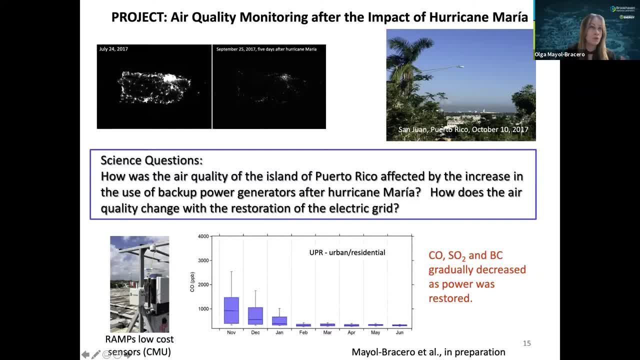 And also Ponce, you know. so the bigger cities, you know, you see them really illuminated. This is just five days after Hurricane Maria, So we had, basically the island was in darkness, you know, because all the electrical grid was down. 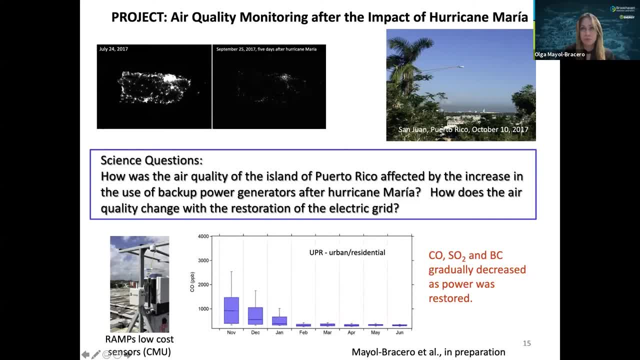 So maybe the lights that you see, there were generators. So this is an interesting story because I was, like, a couple of days after the hurricane I was just running, you know. So you know, there was no power, not much that we could do. you know, the island was paralyzed And I went for a jog And when I was at the highest point of where I live, I look and I saw this haze layer, you know, and I was like eh. 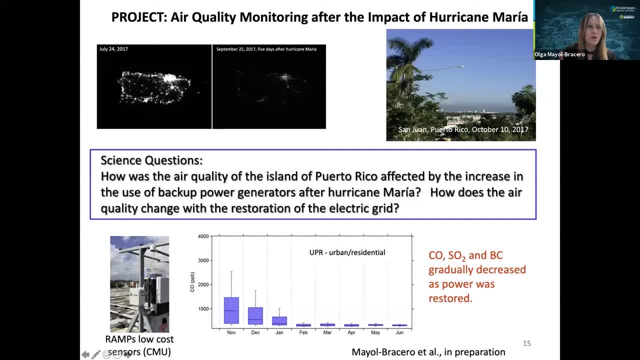 I mean, how can that be? There is no one, almost no one, working, There's no traffic, There's no one you know producing pollution like what we usually do Under normal circumstances. So where is that coming from? And we thought maybe it's the power, backup, power generators that people are using just to be able to have some electricity, everywhere you know, in houses and wherever there is some activity. 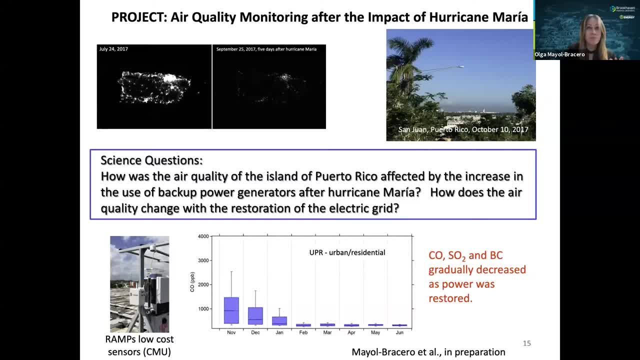 So we wanted to actually study that and that, we wanted to study it, but we didn't have any power in the university. Most of our instruments were broken. We lost them. So an opportunity emerged with the Carnegie Mellon University and they sent us these low cost sensors that they are called RAMS, and we could measure CO, carbon monoxide, sulfur dioxide, black carbon, among others. 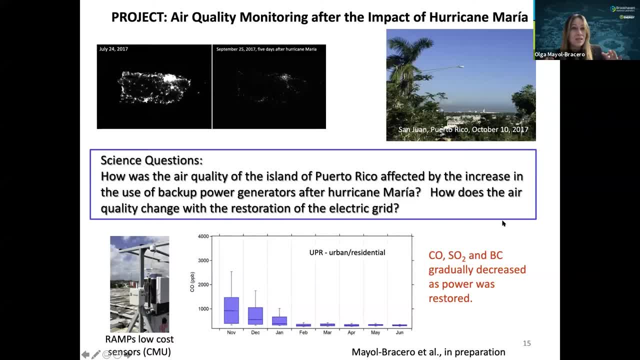 And we were asking ourselves also, once the electric grid start to be restored, what is going to happen? Is this going to decrease the pollution, You know, are we going to be able to show that we're the backup power generators? So, and this is precisely what happened, 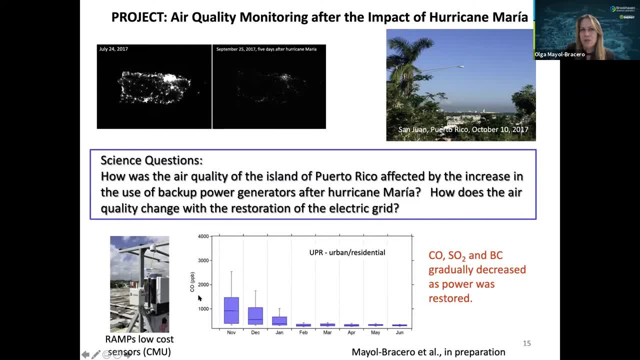 You know, you can see here just an example- with carbon monoxide in November, which is when we started the measurements, and because it was when we got the sensor, and we can see that as the electrical grid was restored, the pollution started to decrease. 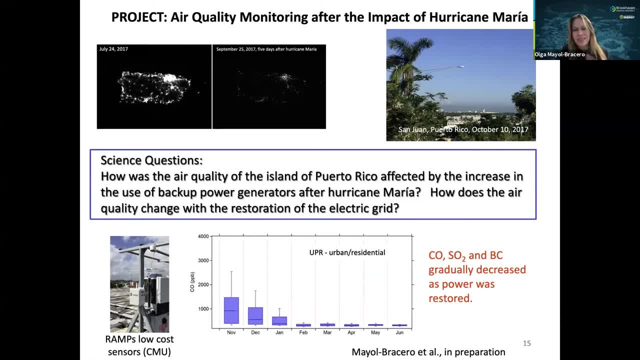 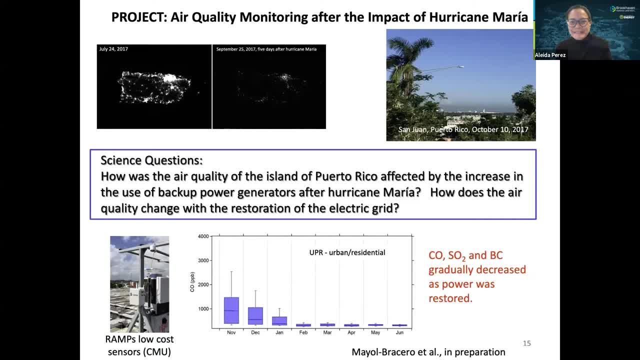 So that was a very good opportunity to show this. That's an awesome data, because you said before: you know, we don't think about those power generators because they're so small. right, If you, If you, You know, if you can have any kind of largeinge? this is is these things? 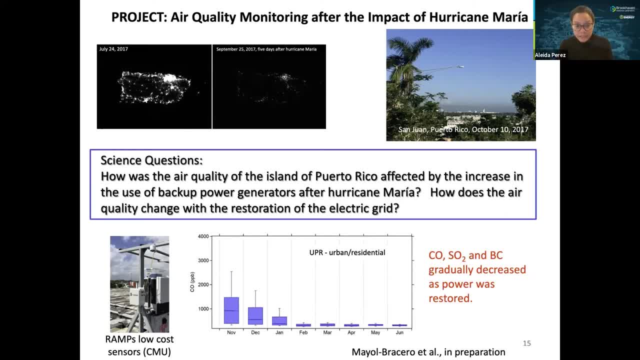 This is and density right. And this is size and density right, And this is size and density right, But they do make an impact. But they do make an impact. It does takes an impact Into our environment and in the air that we feed. 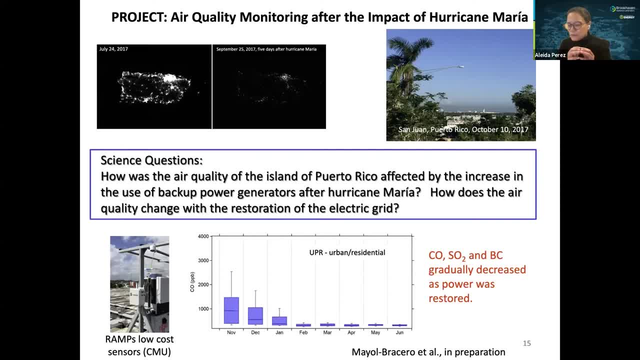 We are getting to the 430.. Now I would like the Cecilia now have some questions about your career path. But before we moveI just want to You know that you have done a lot of work in Puerto Rico and the Northwerks. 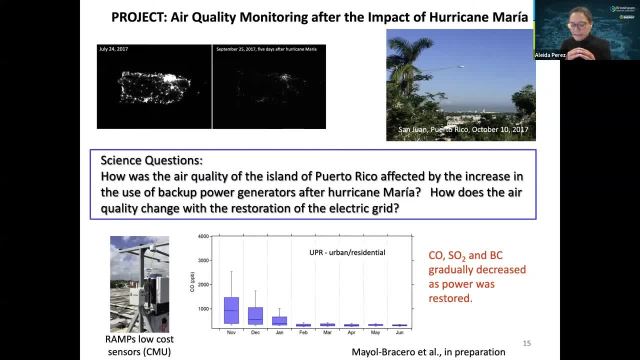 I like knowing about the science, You know. You know you want your kind of stuff. You know, just keeping trying, I know You know I can see what you have to offer. No excited in, in, in aerosols and climate, and I want to ask you, um, what has been the major impact of 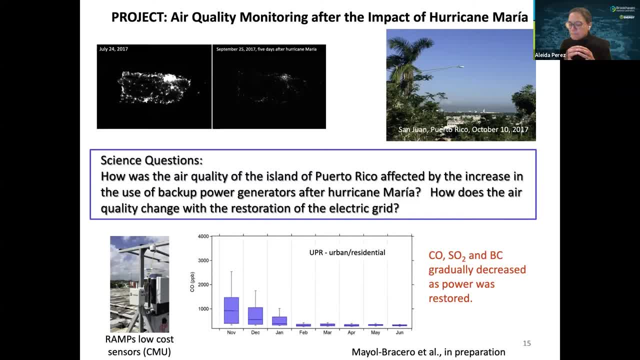 your research in the Caribbean, um, you know, in the tropics area, what has been? what do you feel that is the greatest impact of your or your research in the tropics? and and then you know Puerto Rico and the Caribbean, yeah, so so I think that one of the main things, that that our research activities. 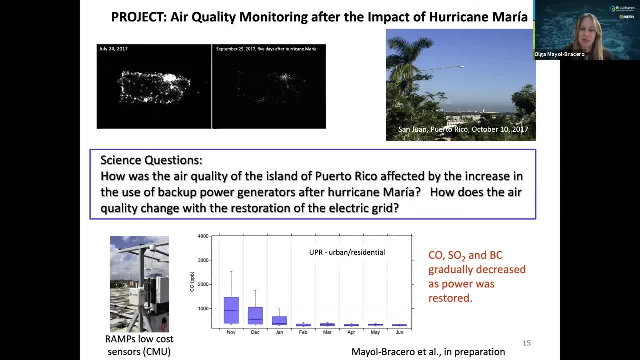 uh, you know, have been able to produce is a better understanding of aerosol types and composition and sources that affect, that are affecting the, the Caribbean region and all their tropical regions, and also I mean what it is, what is important about this, about knowing the type of the others. 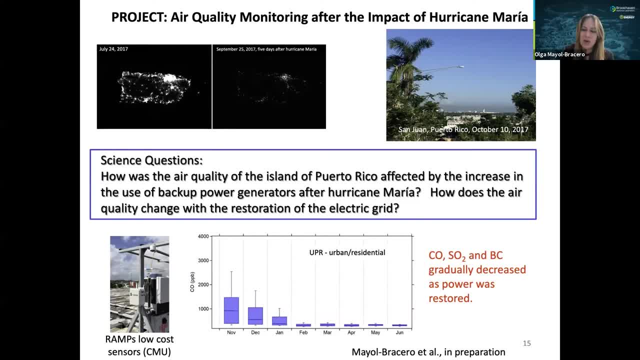 that helps you to to gain a better understanding of of these and the impacts of these on, for example, weather, climate, public health, cloud formation. you need that information about the, the composition and the type of viruses to be able to understand this. you know so. so for the tropics in. 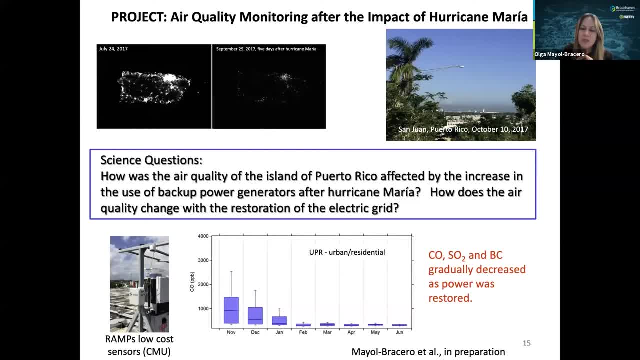 general, you know that. but if we go to to more specifics, you know, like in Puerto Rico, for example, I think that what you're seeing here was a very good example of of something that we learned. you know, this is not the first hurricane that we have, you know. we have had many. of course, no one like Maria in the last 90 years, but we 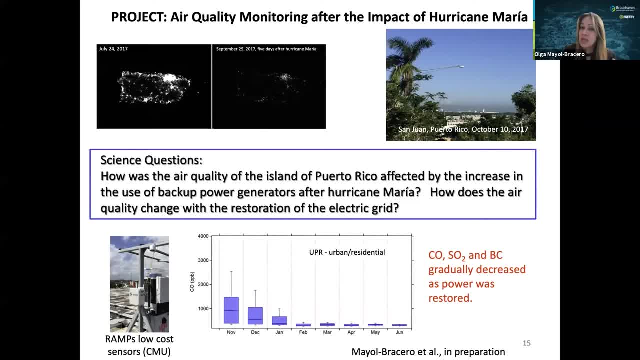 learned that, that these generators are producing a lot of pollution. so you have to be careful in the use of them, because people can die actually out of a poisoning with carbon monoxide, for example. you know you can get intoxicated with this pollution. so so it. that's one thing, that's one aspect, but the 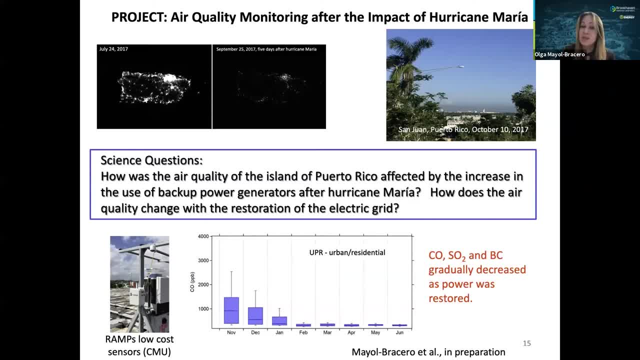 other. I think beautiful aspect of this is how these low-cost sensors they help to to fill in the air quality data gaps that we were having, because our air quality monitoring from the government the network was down was completely, basically destroyed and these low cost sensors gained some data and that that we could use for that. so it shows that they could be deployed in. 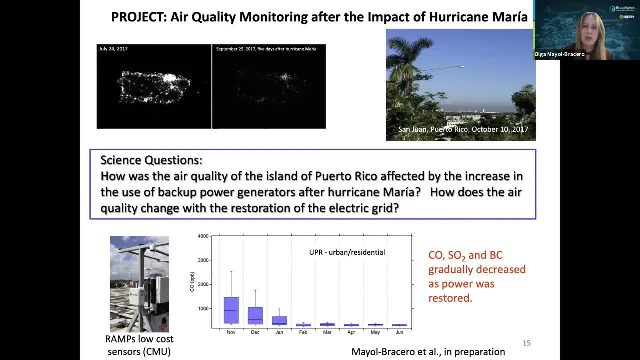 other extreme events or disasters, you know, and they will help in this regard and that's one, you know, one of the things. I think that. another one interesting: we have done a lot of work with African dost, with Saharan Dost and uh a that does comes from Africa and arrives to the region and we're 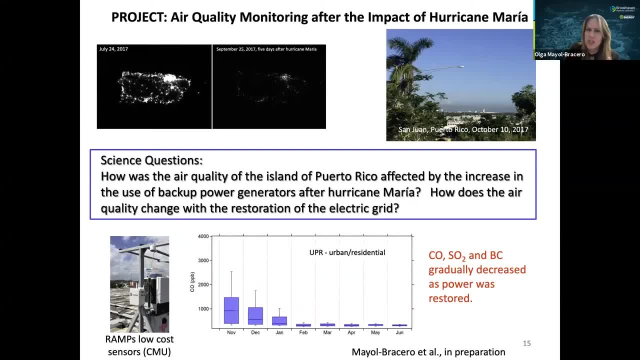 know billions, you know of tons of of dust, you know, and that that does actually, people will think that, well, it does affect visibility, you know, and there are a couple of impacts that we will not have the time to talk about that today, but, um, people will think that their properties would be very, very 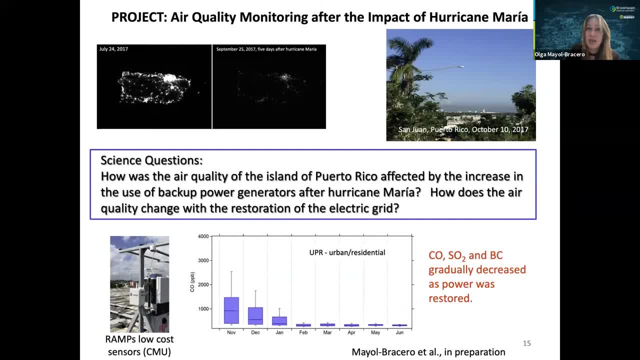 different from the source because they have been traveling, uh over, you know, in the air, in the Saharan air layer, for for days, for seven to ten days, and actually they travel in this layer that keeps them, uh, quite similar to what was emitted at the source, and this is also one of the interesting. 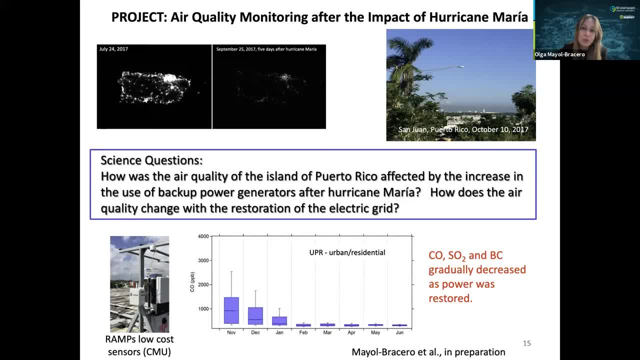 results, that that we've been able to, things that we've been able to learn with our projects. it's awesome, i think you know, like you said, it's uh learning that, understanding the science and the chemistry of those particles you may have understand better. you may have understand better. 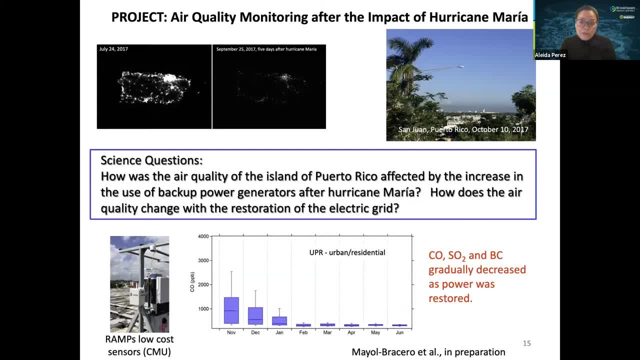 the impact that it has on our health. also, the strong, you know, storms are getting stronger, and so also helps to inform our infrastructure in our places into how better um manage those, those, those events. um, oh god, this has been very interesting. we're good at people to the educational piece so we can give some time to our students, but um uh, 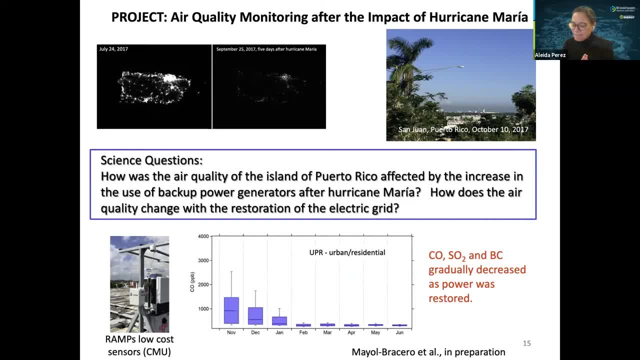 so we have students watching today and, um, did you always know you wanted to be a chemist? say that again, sorry, i couldn't. did you always? did you always? did you always know that you wanted to be a chemist? actually, not, you know i? i when i. 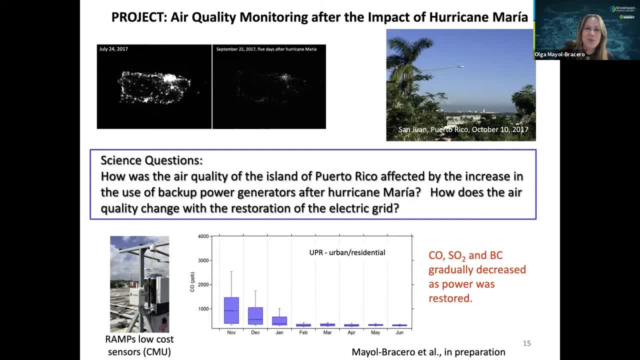 was in high school. uh, i remember i watched a movie- uh, the deep. uh, and after i watched that movie i thought that what i wanted to do with my life was to become a marine archaeologist again. so i i really wanted to pursue that until my first year in the university, at college, when i took biology and chemistry. in that first year i decided that i wanted to be a chemist, you know. so, yeah, yeah, there's a question on the chat because, um, now that you mentioned that you're a chemist said, how does someone with a physics degree play a role in in research that you do? i hope i have. 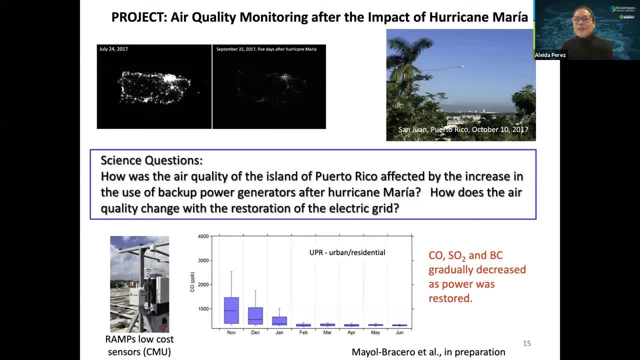 always been interested in atmospheric science, but thought that you needed an atmospheric science degree to do the work that you do. actually, you know what that? um, there are a lot of people that comes from physics in our field and, uh, many people you know that their bachelor or master or phd was. 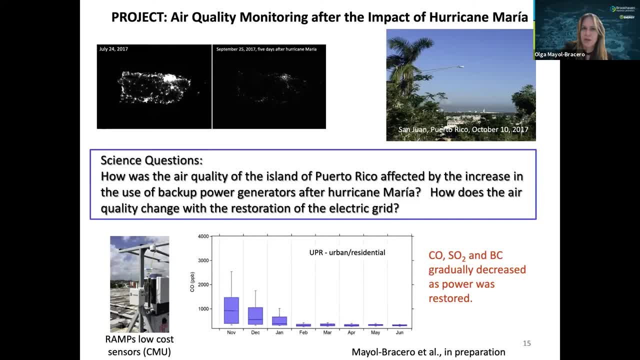 in physics and then they follow up on on, you know, careers in in atmospheric science. so, but you know, when you you do your bachelor's degree in physics, you know um, you can, um, you can become a professor of physics in other fields. you know you could be also that you do your. 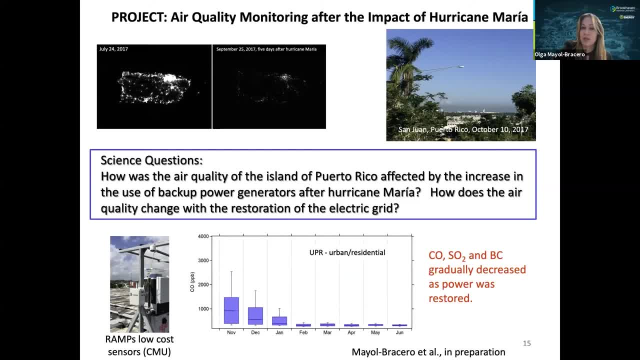 bachelor's degree in physics and then you know, go to to do something in atmospheric science. but your the background in physics helps a lot to understand many of the aspects that we deal with. talking about atmospheric physics, you know there is a lot uh of that, you know. so it's not. 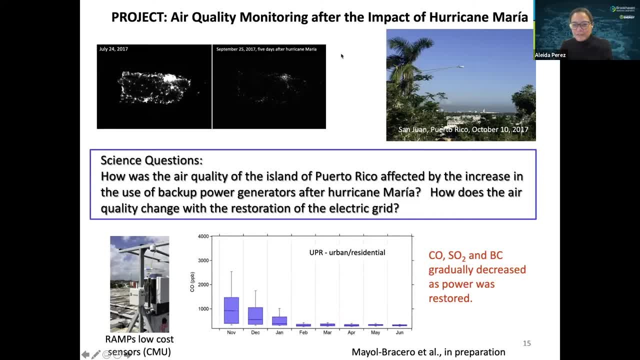 it is possible, you know it is possible and and to that process, that job, um. so i mean, you see myself, you know, i, my degree was in chemistry, you know, and i got involved in this and and you, you know, actually my bachelor degree was in chemistry, my master was in chemistry and my phd was in chemistry, so i did not actually have um. 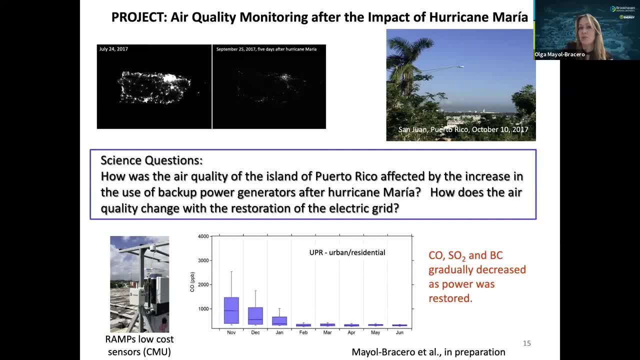 studies in atmospheric science. but my postdoc experience, which was for three years, you know it was in pure, you know, atmospheric science, working with atmospheric aerosols, and i could use all that knowledge in chemistry applied to what i was doing in my postdoc. so and then you 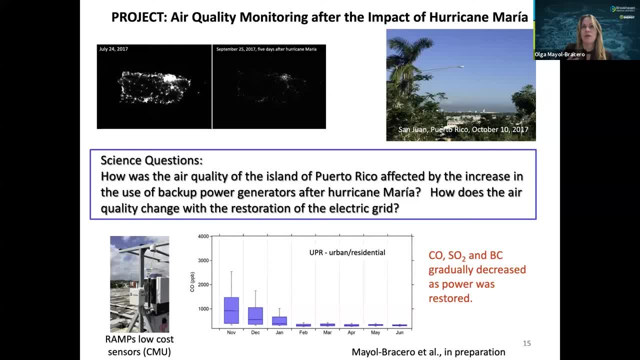 know, you actually become sort of like you know, very proficient in you know, like an expert in the area because you're working so much with that you know, so so you can. you can be also having a background in physics. you know and can follow up on this. 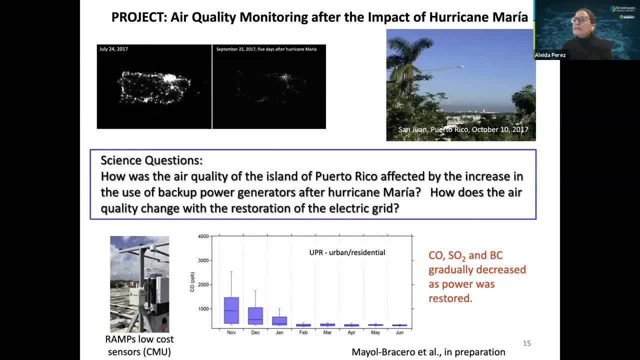 mm-hmm, uh, one thing that, um. the second question that i'm going to ask now is: uh, it's related to- before i forget, um, it's not related to career path, but it says: in times of emergency, since generators are producing pollution at a haste, what are some possible alternatives that will keep people safe? 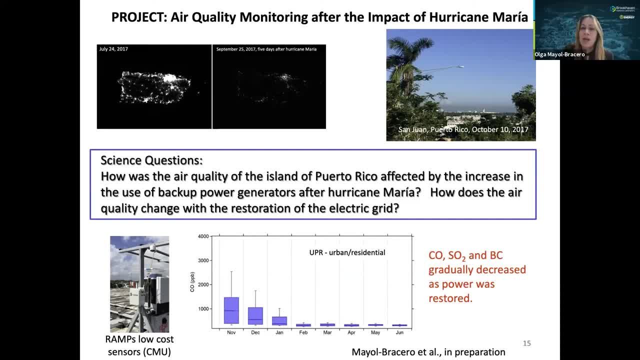 when the power is out. yeah, well, i think that, um, it's not that we are not going to use the generators, you know. it's just that we need to be you, we need to know how to how to use them. you know, for example, in puerto rico, we knew of cases of people that they put them in the backyard, you know. 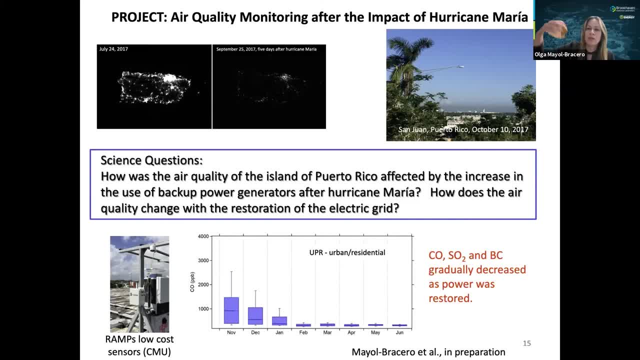 they put the exhaust to the house of the neighbor. you know so, because they didn't want to get the exhaust, you know. but the exhaust fumes, you know, but you cannot do that. so you, what can you do? maybe s able to use the exhaustR, but you cannot do that. so what can you do? maybe you just let's say: you know, you put down two� 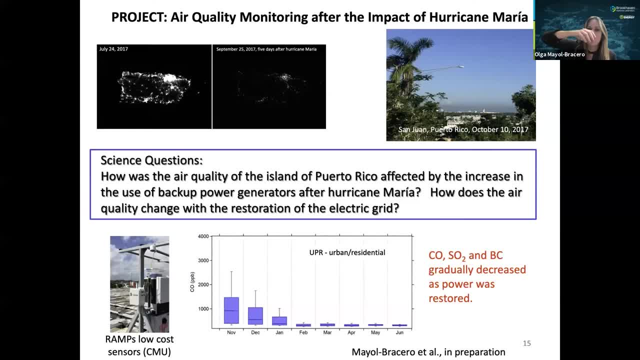 Maybe you have to extend- you know- the exhaust in such a way that you don't get that air stagnating- you know there- and doesn't affect your family but also other families. You know the same with industries, you know. whoever is using the backup generators, we have to know that they produce a lot of pollution that is harmful for human beings and that we need to somehow try to minimize that. 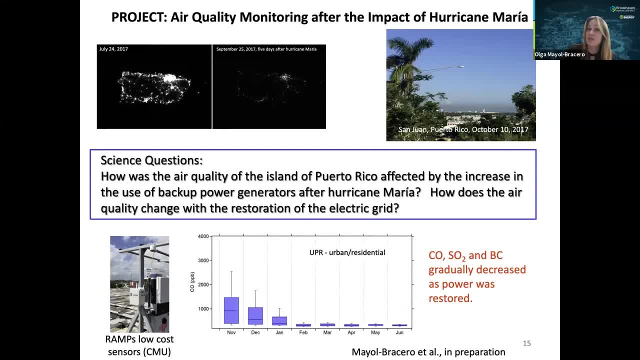 So that is, if we go for diesel and gasoline generators, which are the most common and the more affordable. you know. but you can. you also have other options, Of course. you know you can. You could use a. you could move from your house right to have solar panels. you know that you depend less on fuel combustion. you know and other, you know alternatives. you know. 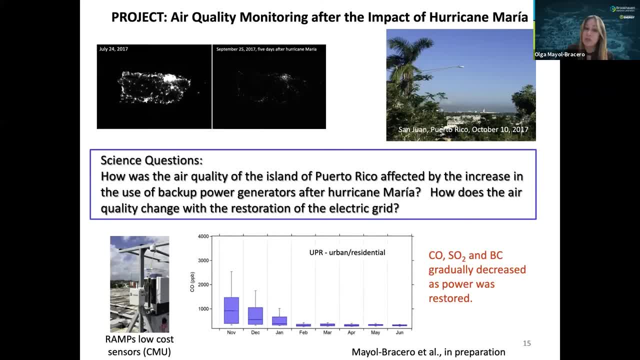 So in Puerto Rico there was- and I hope still, you know, we keep moving in that direction- A lot of people that they got conscious because we were for months. I did not talk, you know, about this in detail, but we were for months, you know. 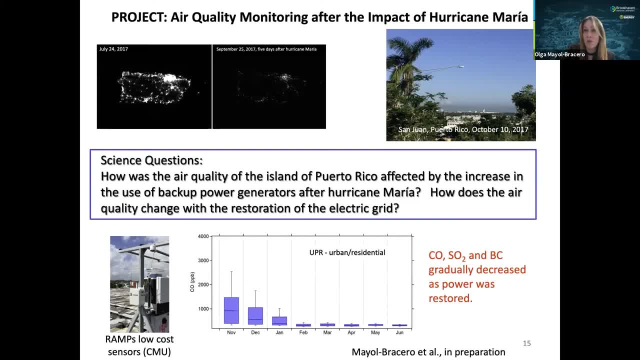 I know people that Maria, Hurricane Maria, was in September and I know people in Yabucoa, which was the area where the hurricane came in, that they were without power until May. you know, almost a year, you know. 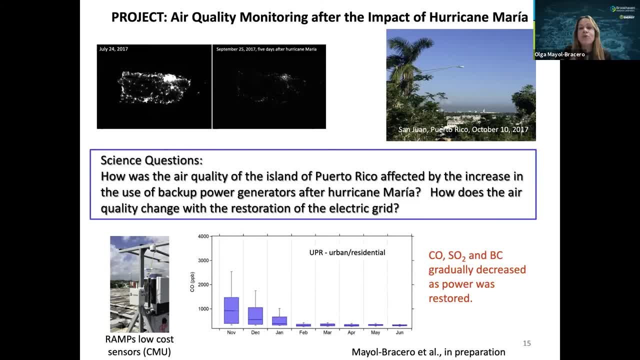 So when that happens, you know you have to rethink how are you going to do things, And many people you know put solar panels in their houses and other alternatives that, as I said, will Reduce our dependency on fossil fuel. 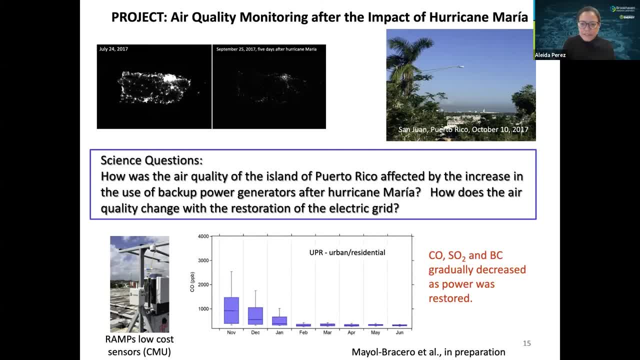 Awesome. Thank you, Olga, And I'm just going to give it back to the career panel. Just didn't want to miss that question. There's a question on the chat: How long did it take you to obtain your degree? So yeah, 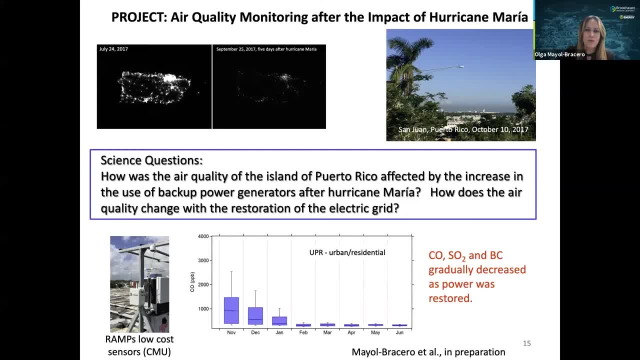 So bachelor degree is usually four to five years, you know, and master is like two years, And this was my case, you know. And then the PhD is usually Between five and it depends on if you have done a master or not, you know. so I know, like in Puerto Rico is an average of like six years, you know, I spent five years, but it was because I have already done my master, you know, so it was less time. It also depends on factors such as your research projects and the instrumentation that you're using, but that's an average, you know so we're talking about five, Six, seven, like 11 years. if you want to do a PhD, 10,, 11 years, you know so. 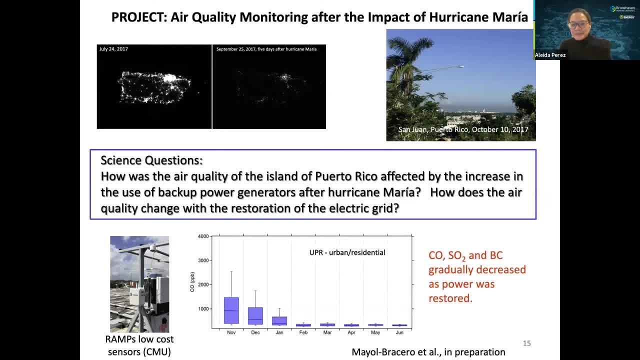 And that's without the postdoc, the training after that too. I know that you participated in the Department of Energy Visiting Faculty Program. How was that experience? Did that play a role in coming here to B&L? Oh, yeah, definitely. 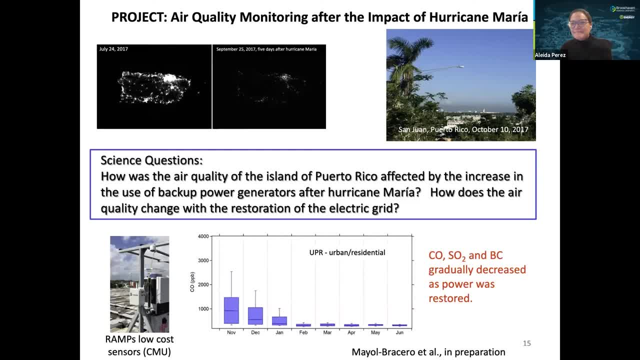 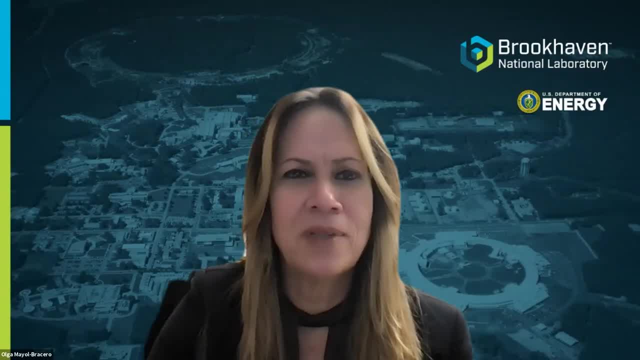 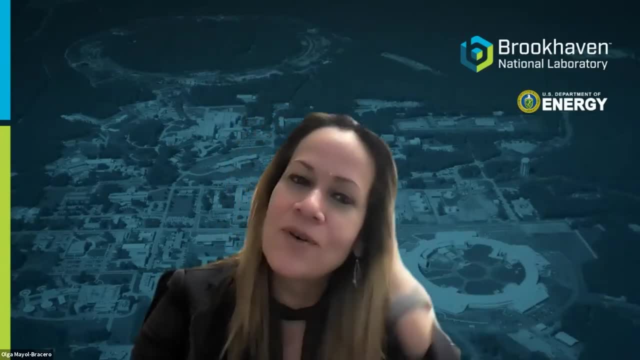 When I was a, probably I should stop sharing my screen. Yeah, so when I was, did I stop sharing? Yes, you did, Okay, okay, So I came here in the summers of 2016,, 17, and 18.. 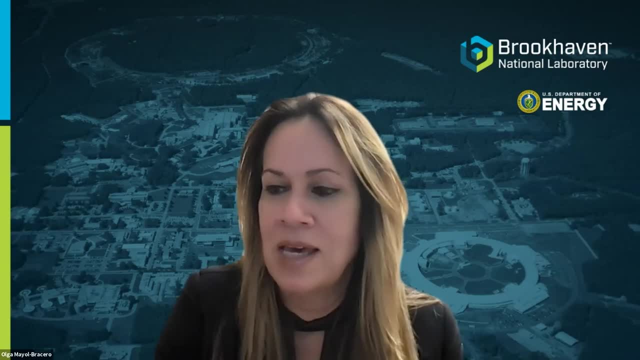 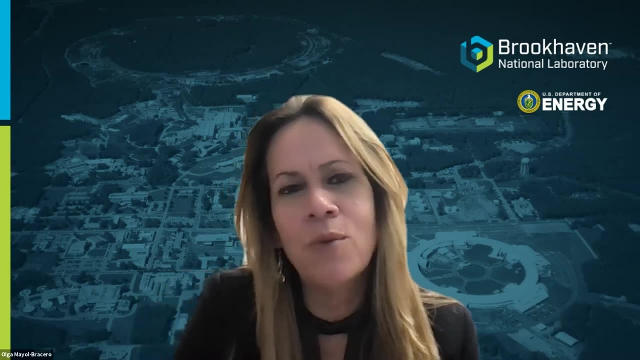 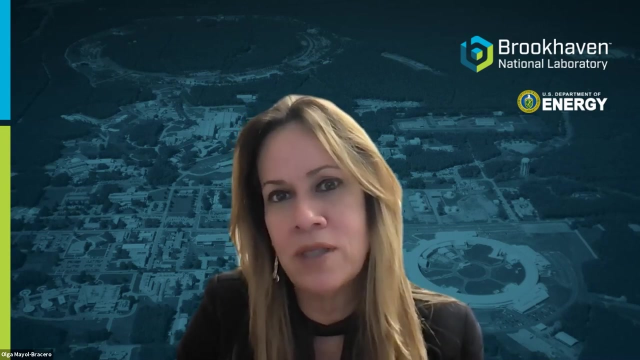 And I came with three students every year- one graduate student and two undergrad students- And we were working with- mainly with- two people here. We interacted with many others, but with art, Yes, Seth Lasek and Ernie Lewis. They are from the Department of Environmental Science, the department in which I'm working right now. 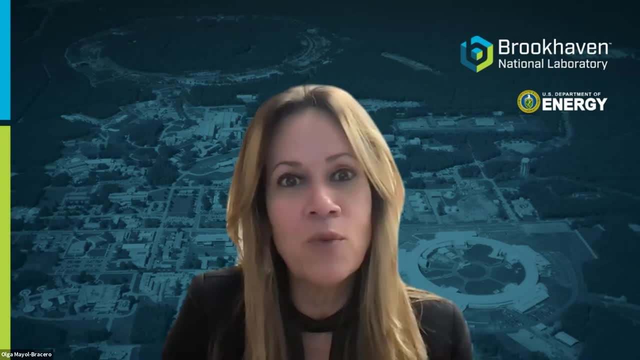 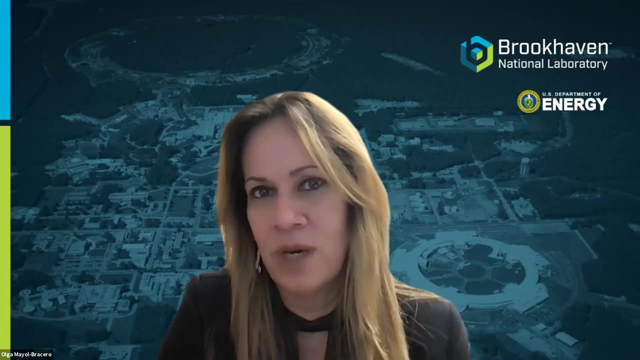 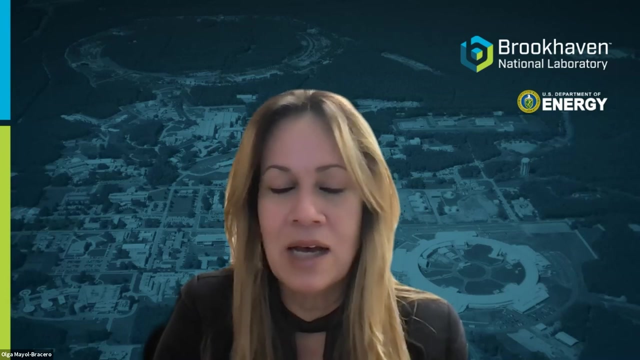 So, and they were. we were working with data from a project in the Amazon basin. It was a project called Go Amazon, So it was a great experience. You know, I get to know the people here, the facilities here And I, when this opportunity, you know, arose, I 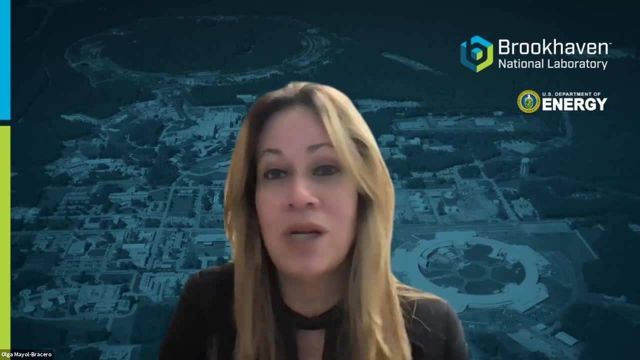 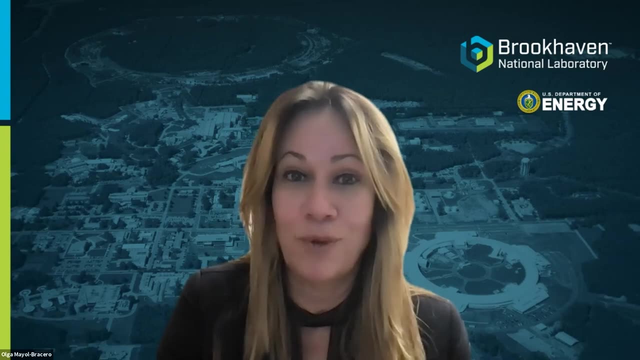 I said, okay, I mean, I know this place. I really would like to work with these people. I know the good science that they are doing, So that definitely had a very large influence in my decision. That's great to hear. 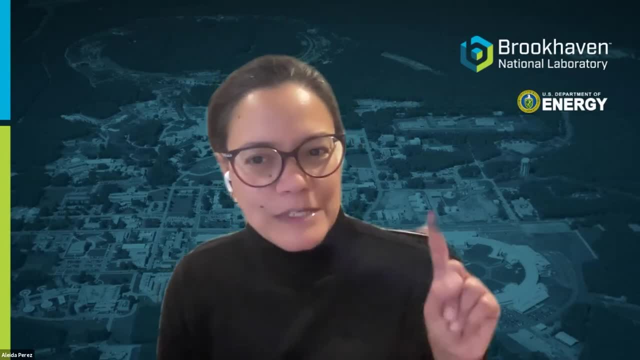 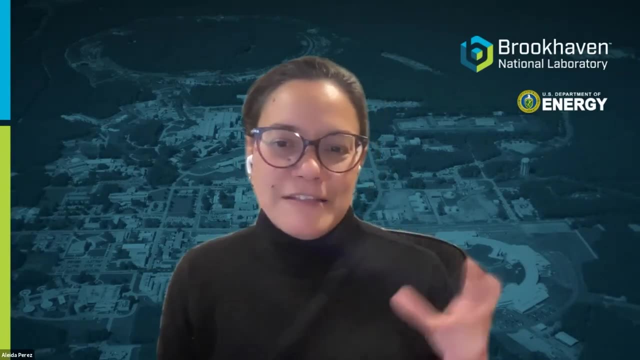 You were. how many you were here. how many summers? one summer, three, three summers, Three summers. That's awesome, Awesome. I know that because you have students, you mentor those students and you're a mentor to them. 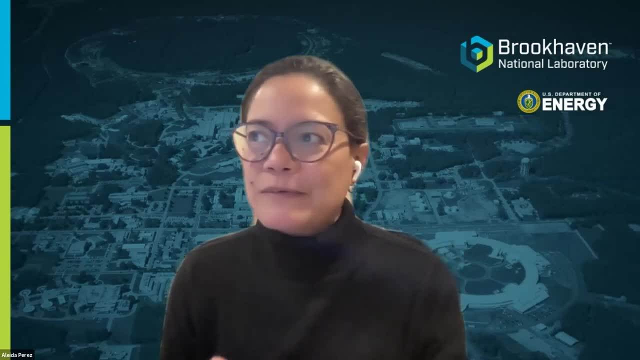 Yeah, How, how important mentorship is, And I you know, for our young students in terms of, you know, finding a mentor and the value of a mentor, of a mentor in their lives, the impact that they make. Yeah, 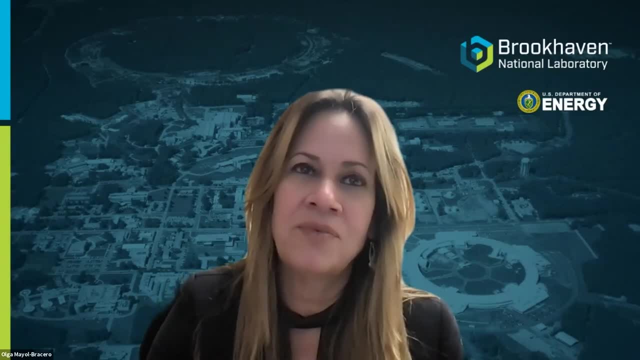 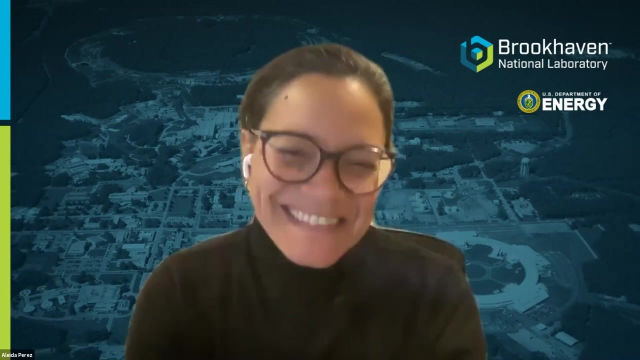 You know, I think that that is very, very, very important And and I had the opportunity in Puerto Rico to to mentor many students at different levels And actually from a high school students, you know that they come to do science fair projects, you know, to undergrads and and and graduate students. 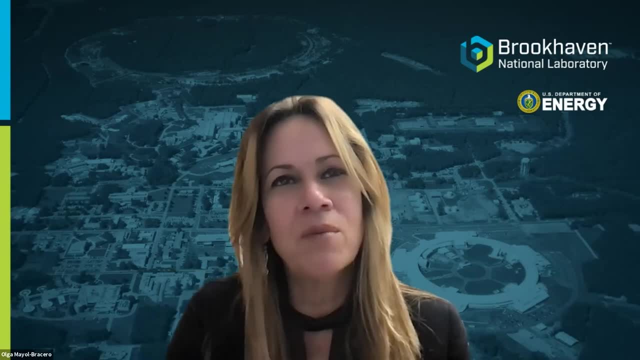 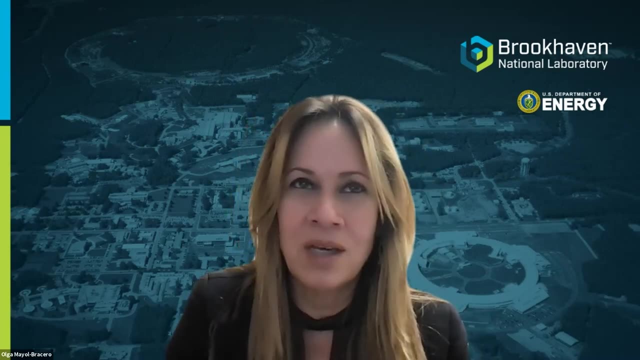 And it was a great opportunity, because you have the opportunity to motivate them, advise them, help them in their decision-making And- and some of them, they might end up actually studying or working in one of these temperatures. Yeah, And they, they, you know- pursue the, the student's dream. 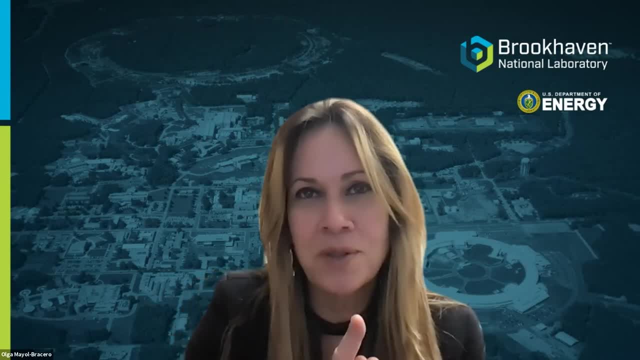 And I, you know, I'm very proud that I'm a student in Puerto Rico. Yeah, And and I, you know, I I like to show that I can help doing this. but I think also I was a little bit afraid, you know, when I was, when I was looking at students. 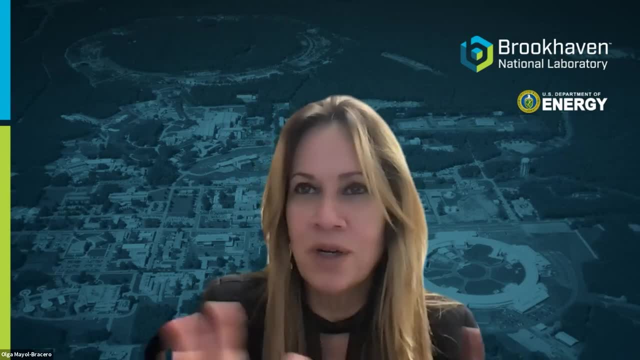 I had a really good friend who was a lot older than me, I think he he did a really good job with, with his skills, Yes, But but, and I, I, I, I, you know. yeah, as I said, I had been studying with, with my, with my school level students and one of the things that I felt I, I, I, you know, I thought I was, I was learning a lot and I ended up coming to school. that was important. 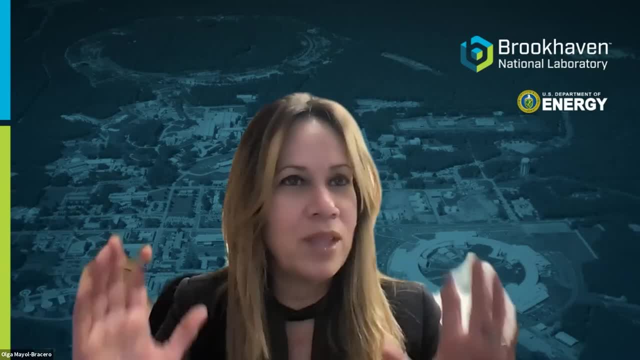 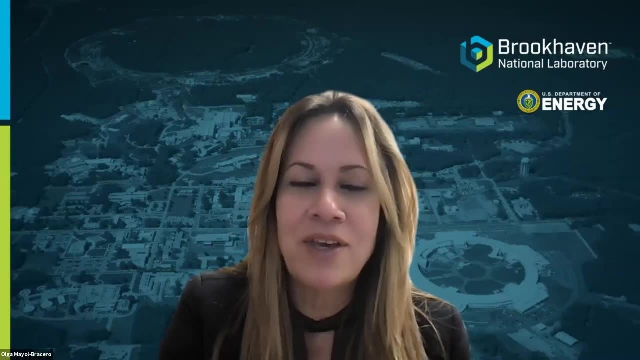 Yeah, science, nuclear, and he was, you know, fixed with that. but he came to work in my group- I was not doing any of that, you know so- and after less than a year he sat down with me and he said: you know what? I think that I'm going to give you some news that you are going to be happy about. and he said: 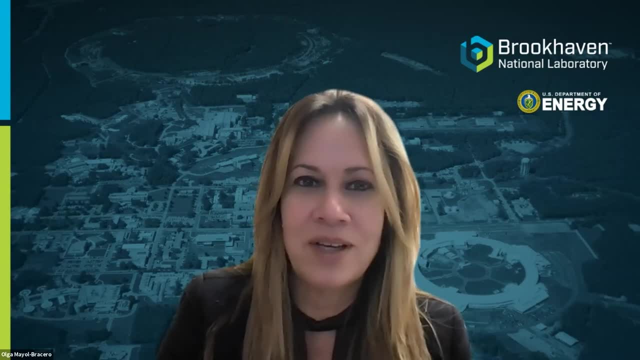 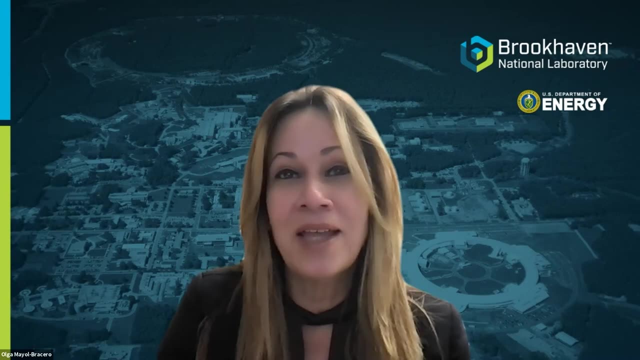 I want to do my PhD in atmospheric science. you know I want to study this and I was very happy he's doing his PhD at Purdue University right now. so you know, and some of my students, you know, I have a student working at NASA, another one at the National Weather Service, with no, and I feel 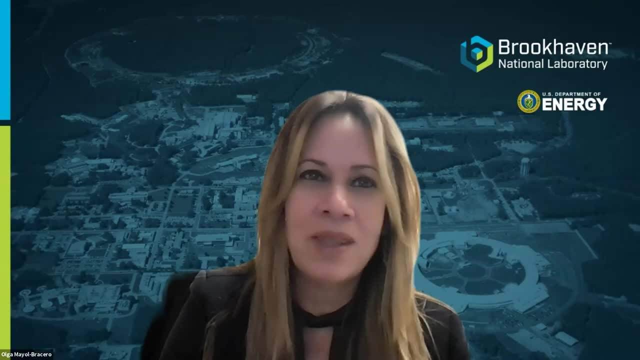 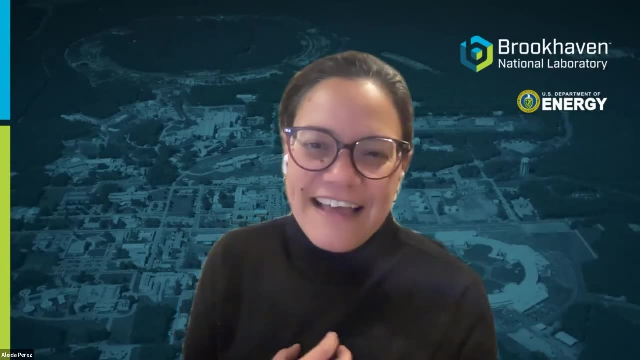 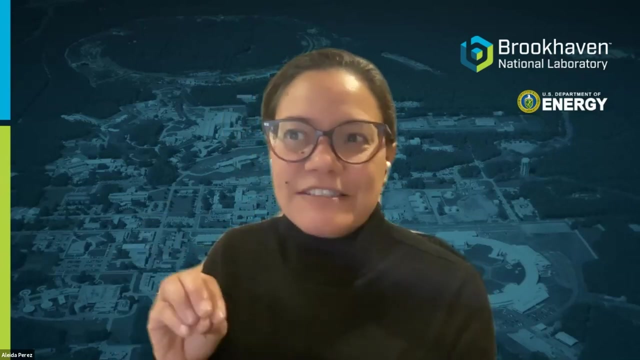 you know, proud of them and happy that I could somehow contribute to their development. so you just spoke with a lot of pride and I also say that it it shows our students that you don't know know where you're going to end up. so taking advantage of experiences like this can inform you. 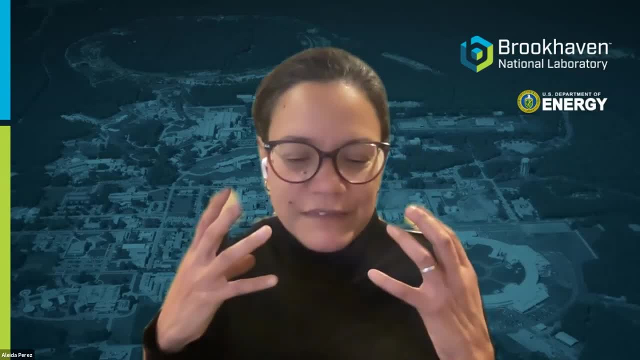 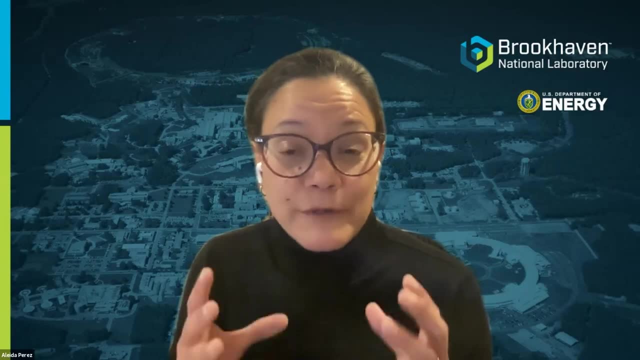 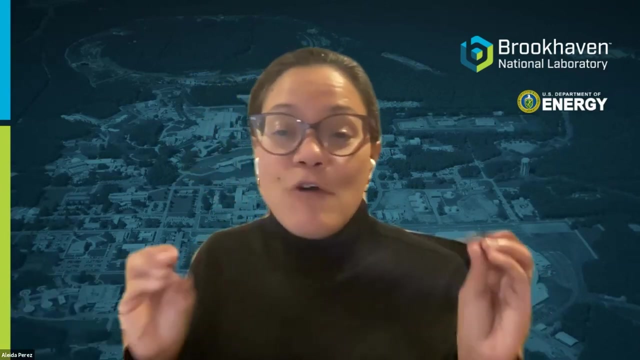 and and, and, and that you and, and you know, inform your choices and decisions. we are a 445 mark. time flies, Olga, when you're having fun, this has been wonderful. before we go, what any? if nobody remembers anything that you said, what would be the last piece of advice? that 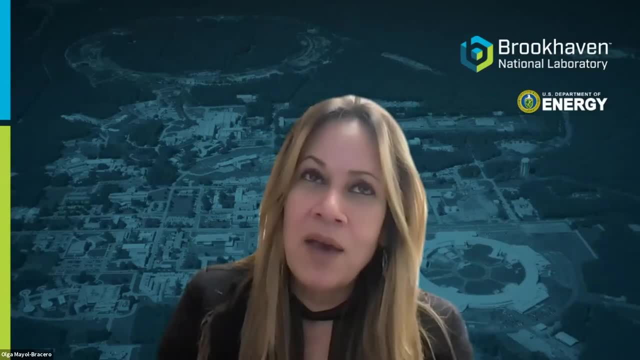 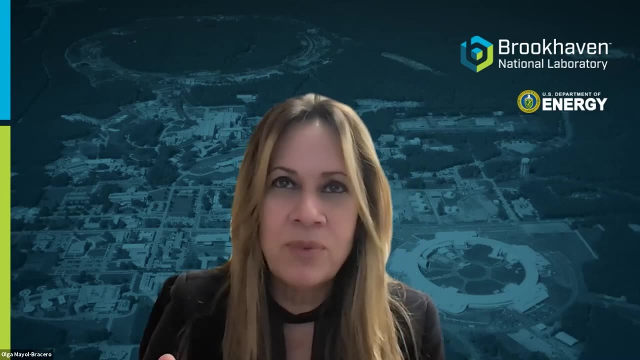 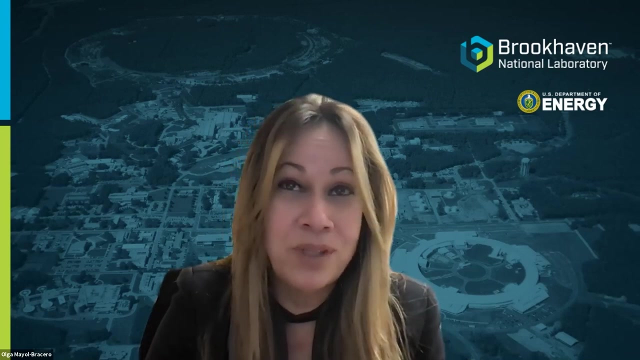 you want to give to our audience. well, I will say, since we have so many students, I will definitely advise students to to get into summer internships, you know, because that will make you a little bit more aware of things that you maybe did not even know, that you were good at those, or